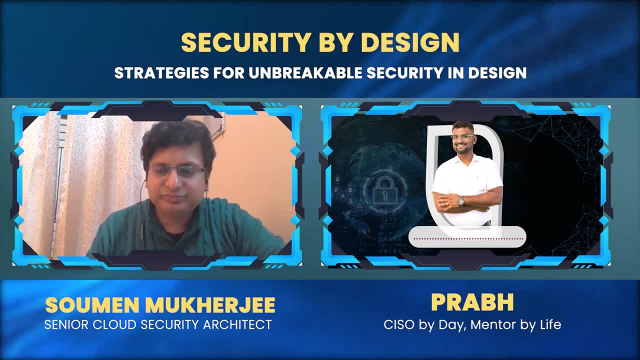 security or making career in secure coding developments, grc, and i'm sure it can be eye opener for you guys and i'm, and if you find this content useful, you know, do reach out to us for more subscribes, links and all that so that you know we can notify you about the new updates. 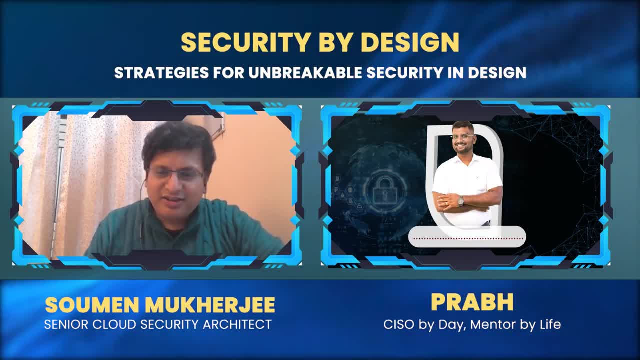 so, dada, good morning, good afternoon, good evening, yeah, very good. good evening, prabh, and indeed it has been a long connection between uh us, i would say uh and we have taken a lot of steps together in this journey of security and i'd like to complete the story that you started. so, yes, 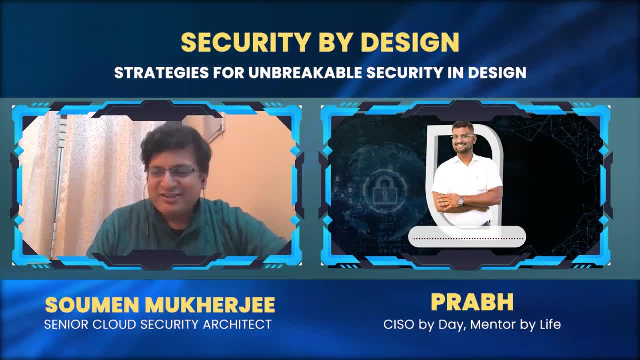 prabh was there and he was taking a cissp session and, uh, actually we were supposed to get another trainer that day, but for some reasons that person was not there. so he came in and he was like he took half of this day and we were like already in his awe and then he said so: 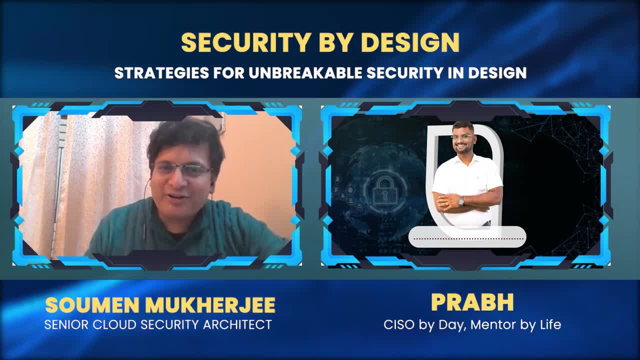 do you think i can continue the session forward? i can teach, and we were like, what kind of question is this? we are like, yes, why not? i mean, there's nothing as such, uh, which prevents you from taking those sessions forward. and i think the next two days were like, really, i still have his notes, uh, and i still have his book with me, which has 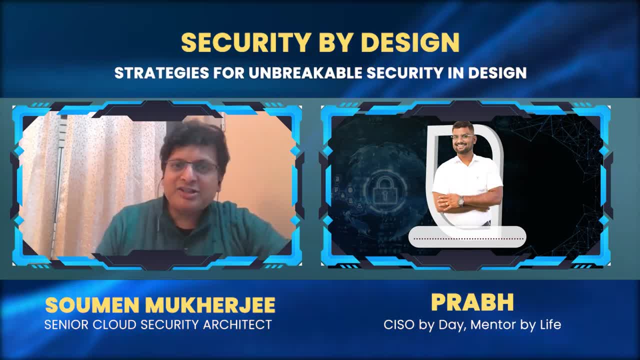 all the markings and everything uh those cissp is is definitely still in my target, but i would say, uh, you know the kind of work that i do it is. it has been a mix of uh technology, security and a lot of hands-on learning. so so far i've been able to. 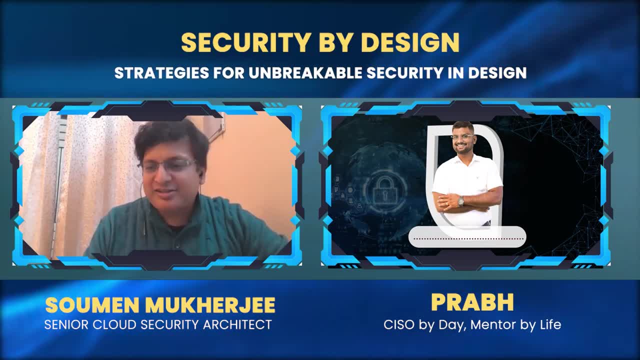 uh, you know, take my journey forward. but yes, for people who are aspiring to make their mark- uh certifications, uh standards, a proper knowledge trainings- they are very helpful and very useful. so that is that is how i would like to start today's session, and no, there is no better person in this community. 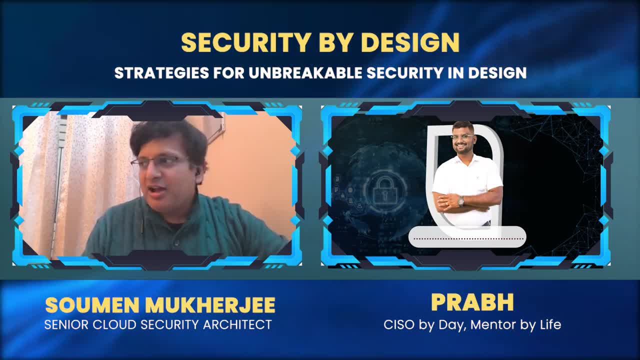 than prabh who can actually guide you in order. trust me, i am in touch with almost thousands of security professionals and i am in touch with almost thousands of security professionals in my linkedin profile and i've seen people referring to prabh's uh sessions, videos from 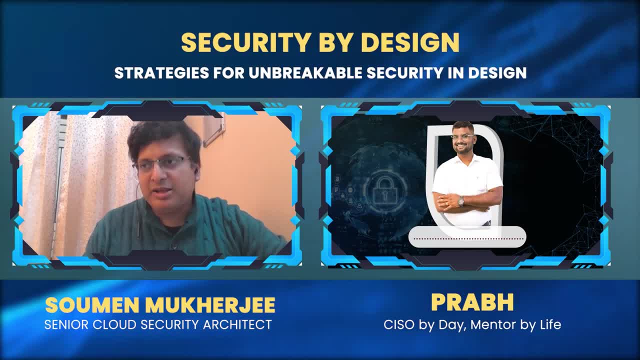 i think almost all the continents and many countries across the world, and it's not really. he's not. he's not a indian phenomena, it's a global phenomena. thanks, it's a privilege to be part of this talk with him and i really i'm hoping i'll take with me a lot of 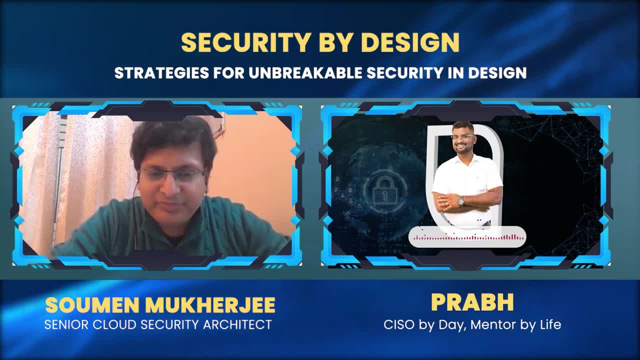 knowledge and learnings. uh, at the end of this session, thank you, thank you so much and i'm and really mean it and it motivated me to make more content like that. but i'm sure after this session, people will be fan of you, because i i was myself as a fan of your write-ups and all that what you. 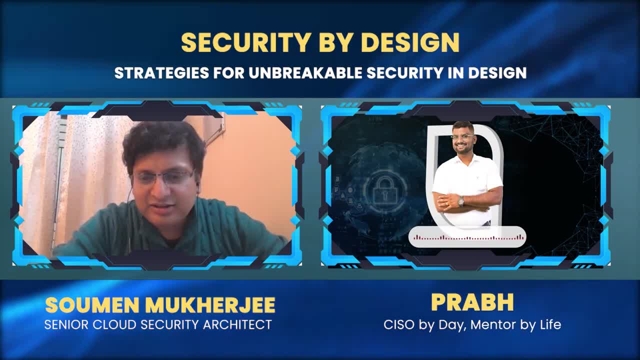 do in architect and all that. so that's why i thought, you know, let me try to have you in this session, and it is, it is a great honor for us, so that today, what is special, what we're going to discuss today? yes, so today we are going to talk about product security, and you know, 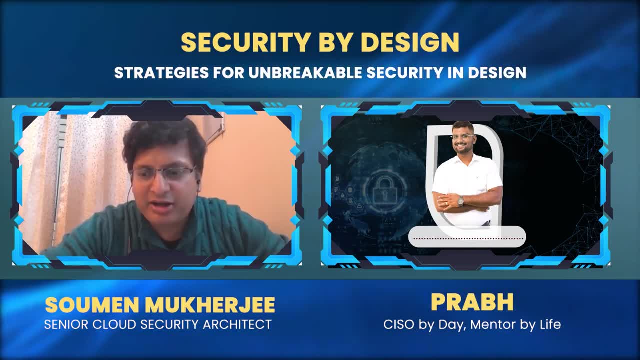 security by design concept in in the in the world of product security, i think there are a lot of people who are actively engaged in software development. you know there are offshore develop. they are working in offshore development centers or they are working in global service delivery centers doing product development for their clients. 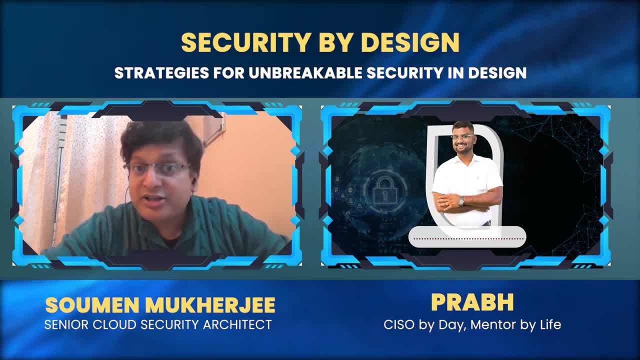 but i still, they understand security, yes, they understand the concepts and nuances of security, but, uh, what i feel is that, when it comes to product development, uh, that is where there are still- there's still a lot of work that needs to be done, because product development, it's a, it's a. 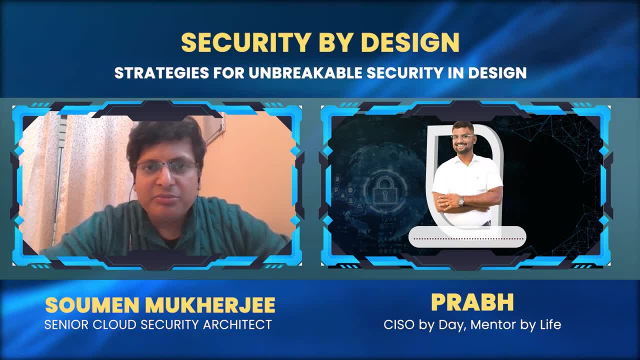 different ball game. it's like, uh, just, it's just like the red ball cricket that you have. you know, everything else is white ball, yes, but this is definitely a red ball cricket. it's, it's a test of performance, uh, patience, uh, and skills. uh, because a product is, of course, once you develop a product. 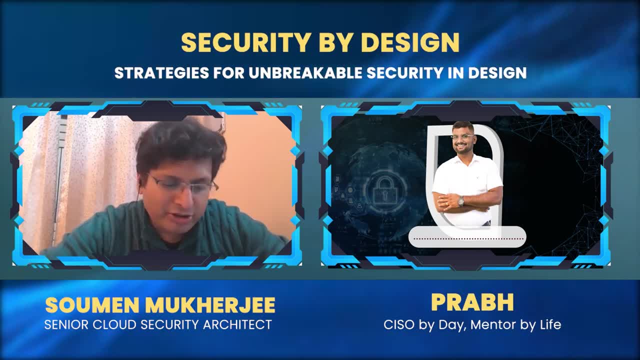 launch a product, it has a pretty long lifetime. i've seen products which are running in the industries for the last 20 years. you know they are being supported, they are being maintained. uh, you know they are getting security updates. so it's not a six months, one year, two years. 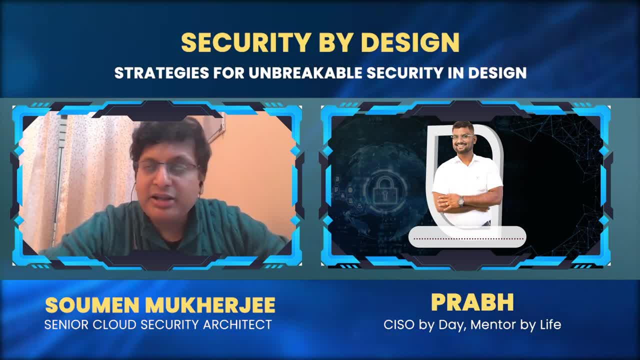 journey. uh, it's a pretty long journey and i think it's a very important thing. i think it's a very long journey and that is where it becomes very important. uh, you know, when we talk about uh product security and one of the uh common things that i see typically uh with products, 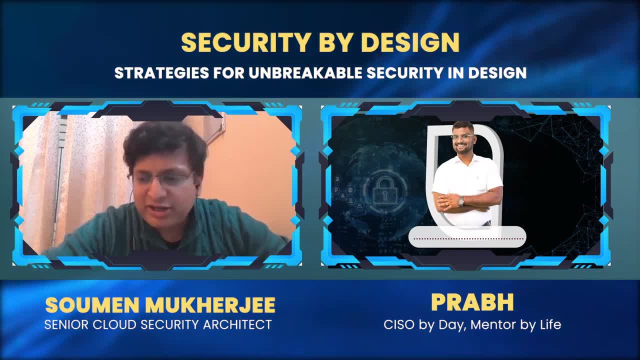 is. you know, when some, some organizations say that, okay, let's develop this as a product, you know security becomes an afterthought, security essentially. you know. just when they are ready they say, okay, let's put it in pen test and let's see what are the results. but 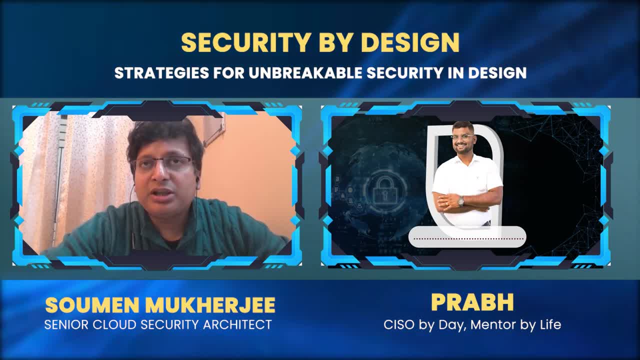 that is, i think: uh, you know, you get a very good pen test results, you get a lot of vulnerabilities and your team says, okay, you know, great, let's fix them. they fix them. but what you don't really realize, that it is just a symptom. fixing that you are doing, you are not addressing the root cause. 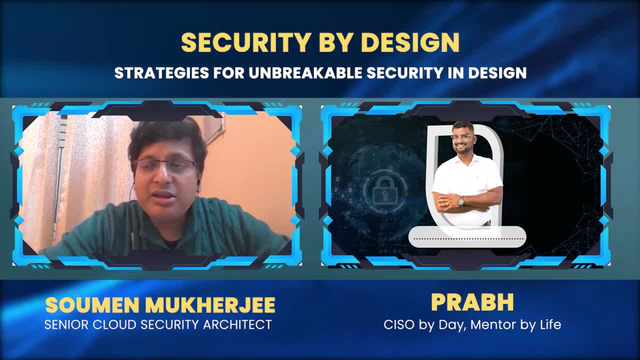 uh, because again, six months down the line, one year down the line, you will end up in the same situation where your product will have another numerous set of vulnerabilities and you will continue to do the pen test. but it is again just like identifying the symptoms and fixing them not. 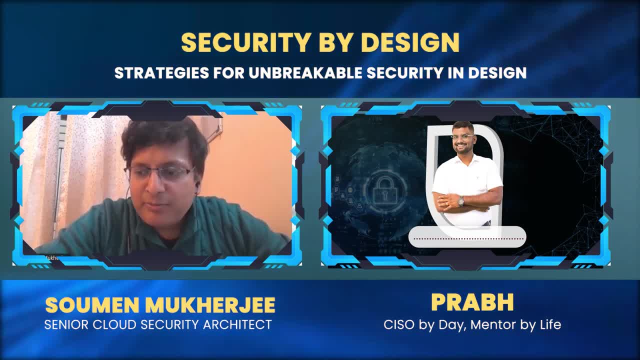 really addressing the root cause of the problem. so what i am going to talk about uh now is basically a model where uh, we can um, uh, you know which- which can basically address a typical product development organization or a team which is developing a software, uh for internal use or even for customers, but it's essentially a product or a service which is 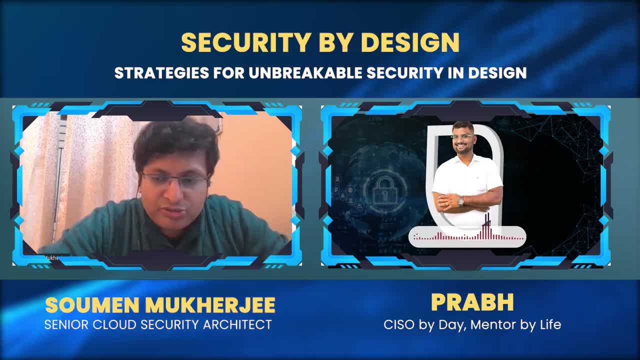 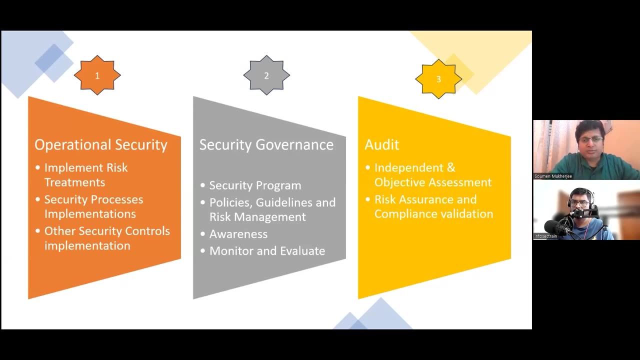 going to be used by the people. that's great, so yeah, so, uh, typically, if i can, yeah, i'll give you the host rights. yeah, yes, i'll just quickly share something. so, uh, typically, when we talk about a, a product security organization, so the, i see like the three, 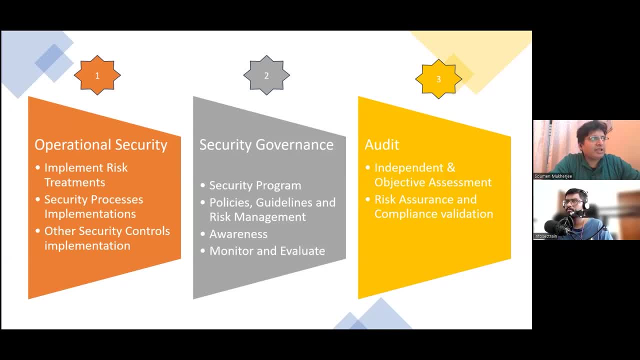 lines of defense, uh, for product security. so we basically call, we can call them, the first line being the operational security, uh, the second line being the security governance and third line being the audit. now, how are they important, uh, what role they have they play in this entire game? is, is, is, is. 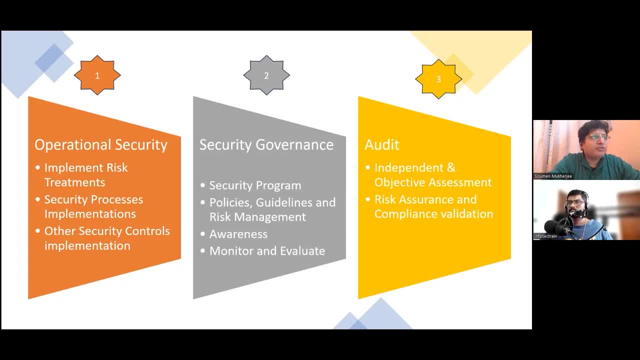 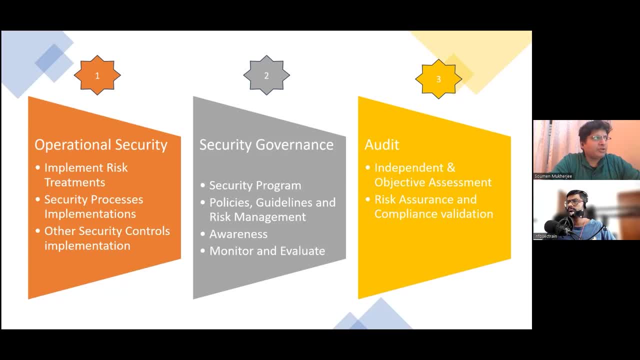 have the you know the product, uh security guys, the security engineers, the uh architects, but essentially that that you know. the full story gets complete when you have all the three, three layers in place and when we talk about the operational security part. so it is more about uh implementing the risk treatments, uh implementing the security processes and the. 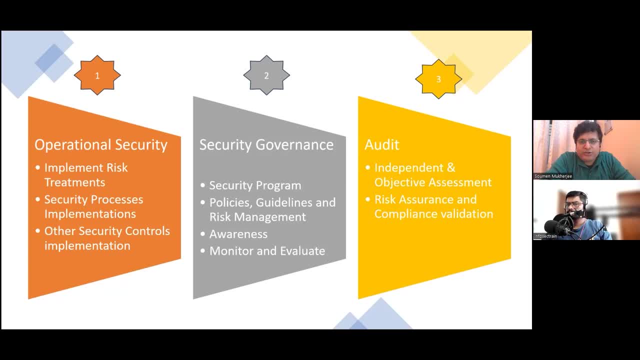 implementations and the other security controls which have to be part of your software development life cycle. so i think, moving forward, we will look a go a little deep into the software development or the secure development life cycle as well, and then we will talk about the security controls. 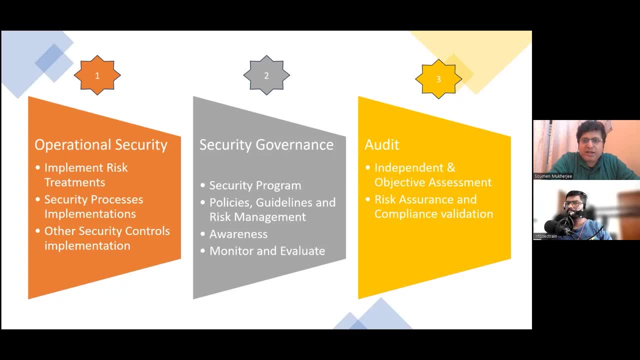 as well, but the operational part is typically something which is part of the r? d teams itself, and that is where they actually are doing security. uh in an out, you know. so typical product security is not a one day thing. it's a journey, as i said before, and it has to be a part of your. 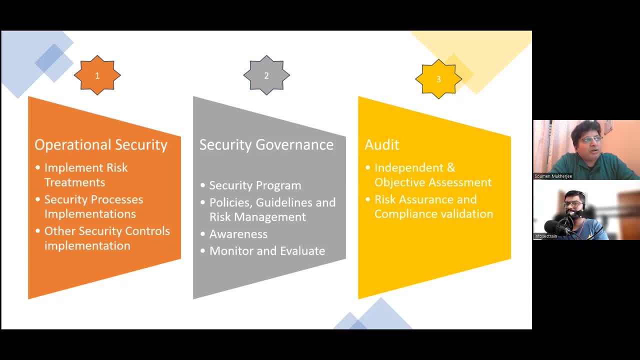 software development process itself. now the next question comes: is that okay? what are the supposed to do? how they are supposed to do it, what are the guidelines, what are the policies that they are supposed to follow? so that is where the security governance comes into play. the second: 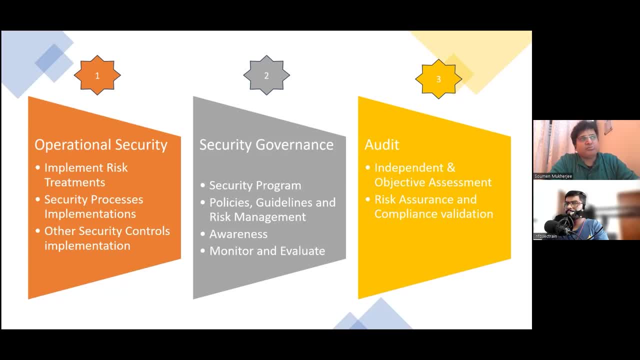 part or the second layer of defense, which is which can be a security office? it can be a product security office, it can be a security governance council or it can be a group of security architects who are collaborating together to share the best practices within the organization. so typically, you have security program, you have a product security program. that 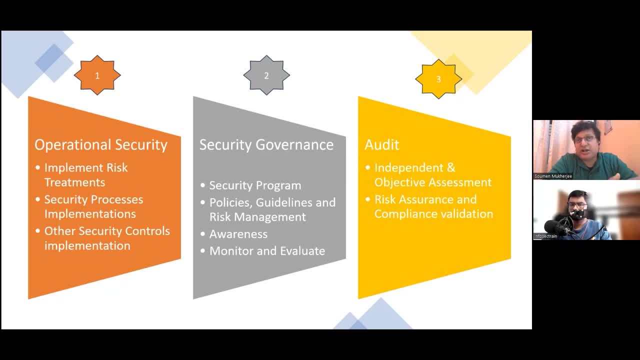 essentially runs, which says that, okay, you know, this is how we drive the product security, this is how we make sure the product security is an integral part of our software development process. so they outline the policies, guidelines, they help the teams in risk management, uh, and they constantly work with the stakeholders for bringing out the awareness. 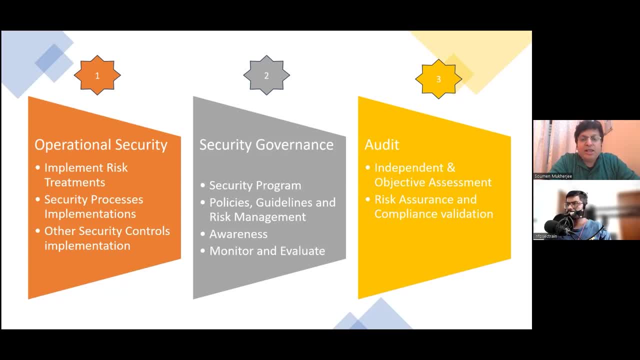 on product security. so typically what i've seen is uh. for many organizations, awareness is all about uh, basically getting people trained on basic cyber security hygiene. but that is good. that is always the first step. but when we are talking about r&d people, then there are 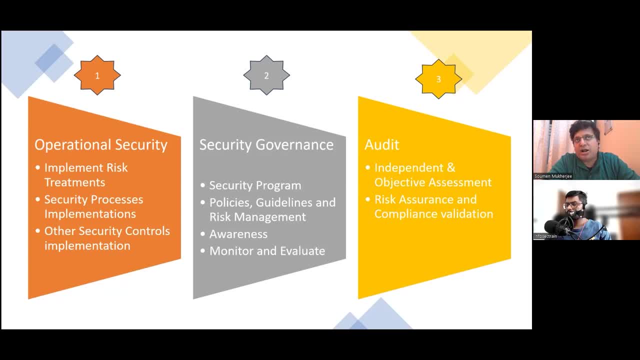 various- uh you know- standardized trainings that you have to undertake, like secure coding, secure uh, secure code review, uh, security scan. uh you know trainings about security tools, uh utilization of uh you know uh essentially bringing out the devsecops culture in the organization. so that is essentially. 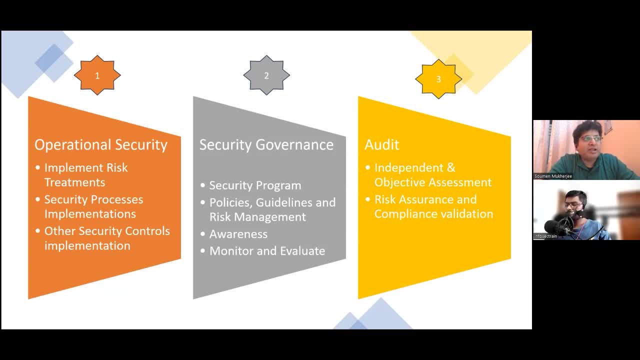 part of your policies and guidelines, And that is where the awareness factor also comes in, where you basically make people more aware of the security practices of you know, building your software development more robust and more integrated with security controls. And, of course, the last part, or the third layer of defense, is where the audit comes in. And of course, audit, as we all agree and we all know, is a very important part And it's an independent and objective assessment right. 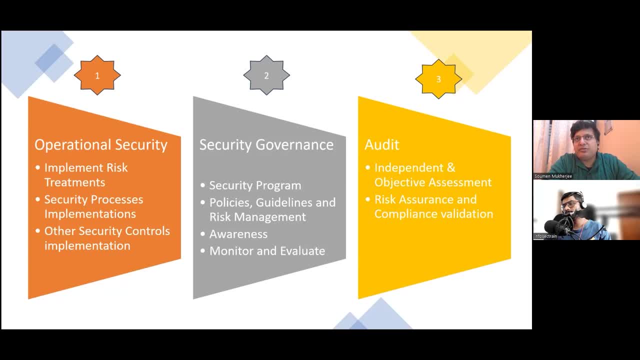 And essentially you always need somebody with a fresh perspective, with a, you know, independent position, to come and look at the security And do an assessment of how you are doing your stuff, how well you are doing, or what are the areas of improvements. you know, that is essentially how it comes from the audit on the audit side. 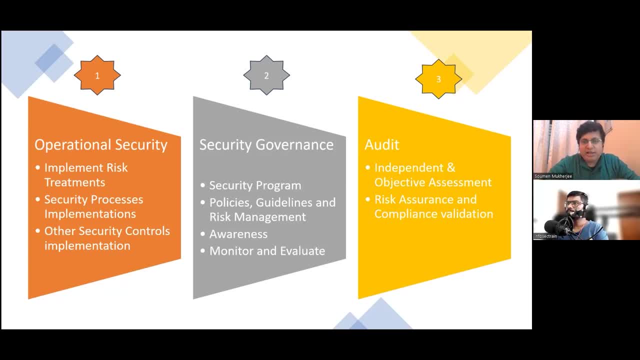 And yes, typically people say auditors will always find fault. but trust me, it is for your own betterment. The more fault defined, the better You will become tomorrow, you know. so I think that is one of the key takeaways. 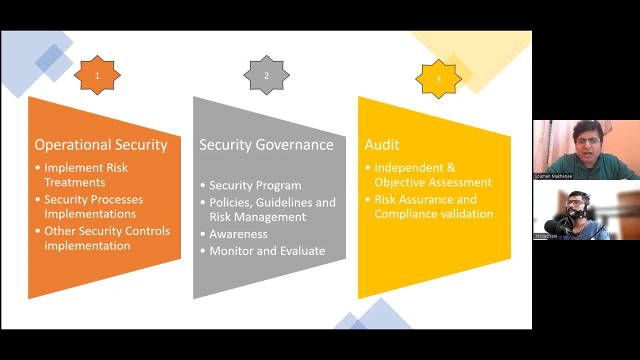 So if you look at this- three lines of defense- I think they cover all the areas, all the aspects of product development. And now we can go a little deeper in in the product development thing. Let's take a hypothetical scenario. I work for the product company. 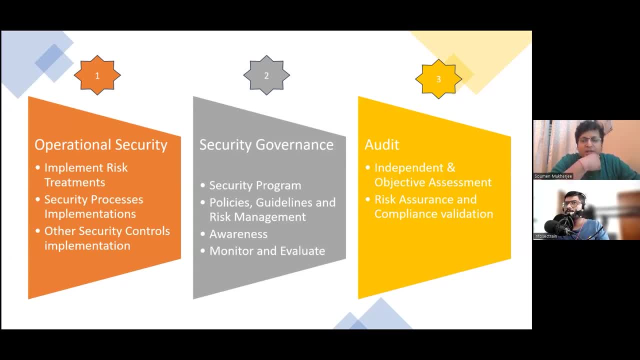 Right, Okay, So when I work for the product company, you know I'm planning to build one, You are a solutions. Yes, So from that point of view, particular case study: like, okay, operation race. So if you can spend five minutes on this area to, with this reference, you know, role of operation security from this angle: security governance and audit. 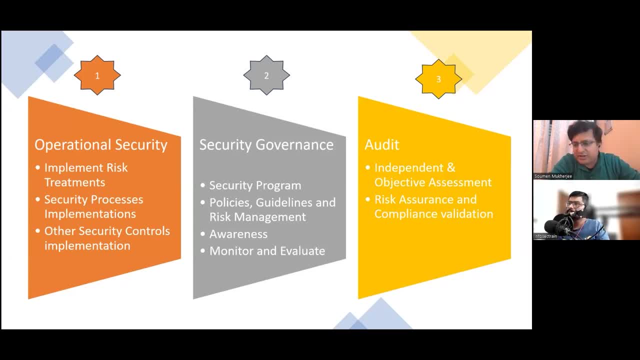 So that gives a new insight on this particular Exactly, exactly, No. I think that's a great example. Typically, when you start developing a software, so you basically say that, okay, I follow a secure development, Okay process, and that is where the operational security comes into picture. where you say that, okay, i would. 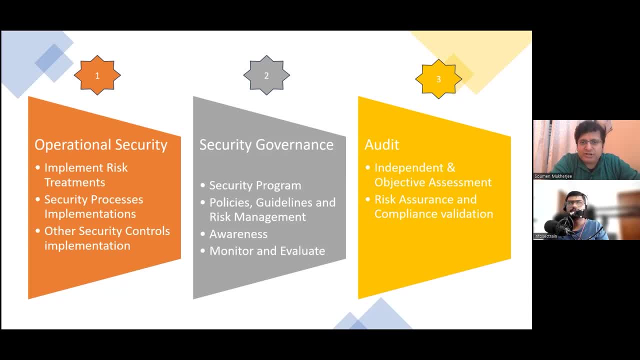 like to have a security champions program. in my organization- that is the security governance part- they say that, okay, let's do a security champions program, let's position some security engineers within the team and let us also have a security architect who has a high level overview of the 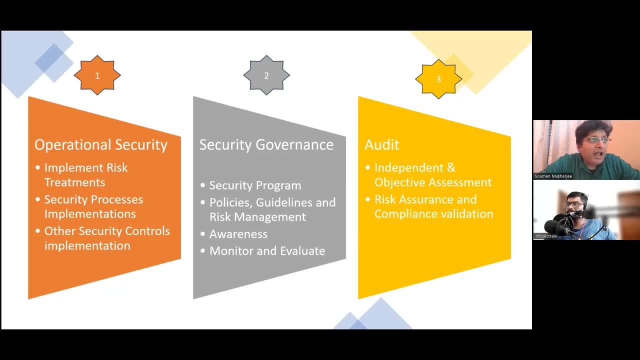 entire end-to-end security and then they, the operational side, the security engineers. basically they become, they are part of your development team, they work with your developers. they do help in the secure code review of of all the code commits that you are doing as part of your. 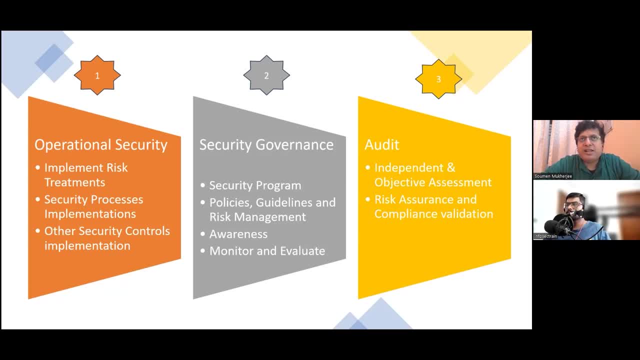 development process. so what you can do is you basically also, you know, typically in most of the organization they say that okay, they follow the four i principle for doing code commits. so what we say that, okay, you have, you have one peer who is a software developer, you have one security engineer or a security architect. 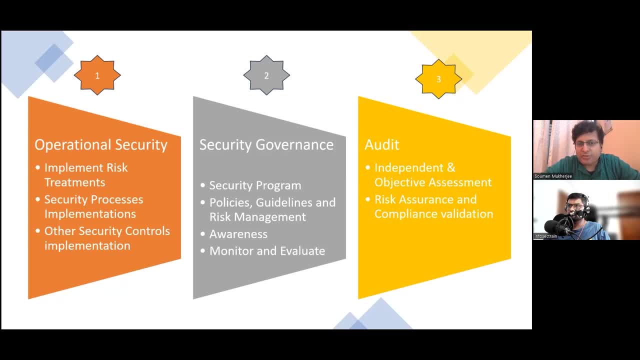 who also looks up your code as part of your code commit procedure, code review procedure. so there is a, you know, functional review as well as there is a review which is done on the code from the security standpoint. and you know, typically when we implement or, you know, go for. 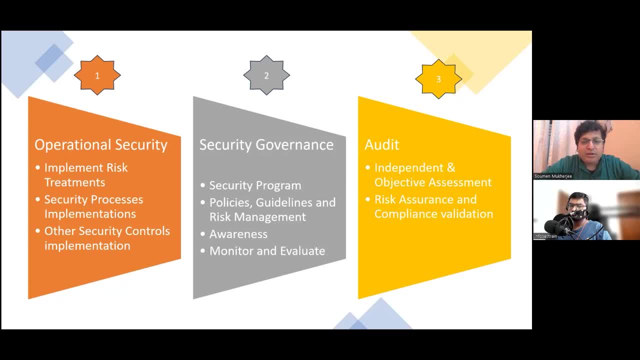 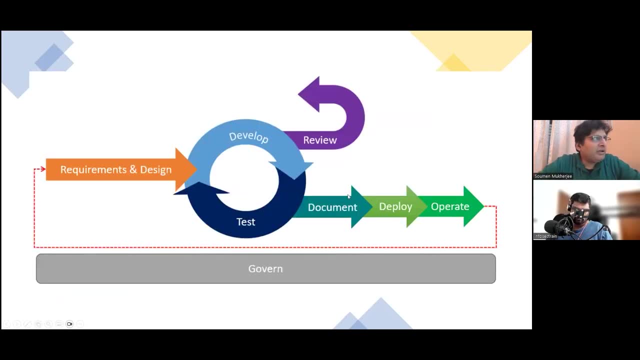 a secure development life cycle. we, you know we can basically jump to the next slide also, and things that, when we look at the requirement and the design phase, you know we have the development testing review, a document, deployment, operation and you know the governance is something which goes all along. 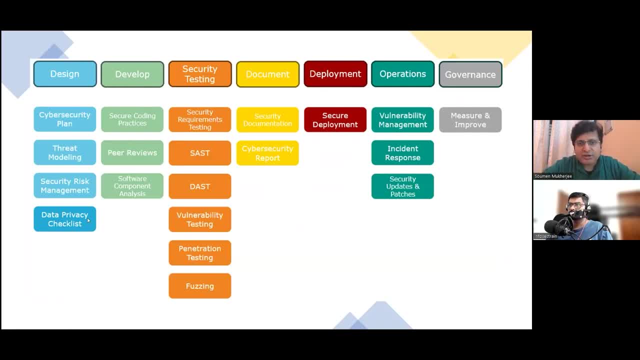 a very if you drill down further in your case. uh, so you know, for in the design phase you have, you outline your cyber security plan and typically for the crm uh example, when you outline your uh software design, you also design your cyber security plan as part of your design. you, you do a. 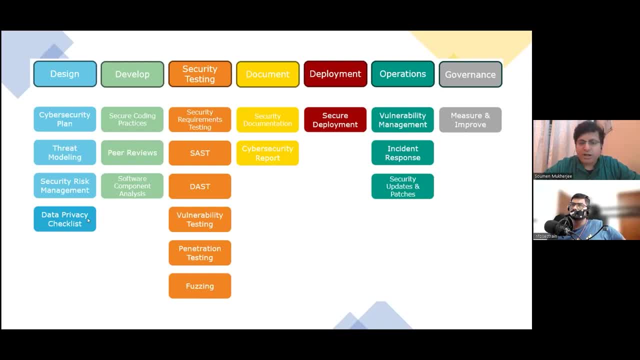 review sessions. so, on the security side, you do threat modeling sessions, you know where. basically, you uh say, okay, what are the threats, what are my end points, what is my attack surface, what are the attack vectors? uh, what are the possible- you know- mitigations that i have. what are the things which? 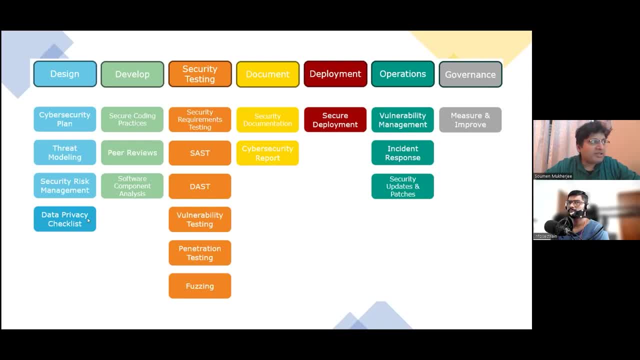 are not mitigated, you know. then, basically, you get into that security risk management. after you do the threat modeling, you say that, okay, these are the things which are mitigated, these are the things that needs to be mitigated. and, uh, privacy, again something which is has to be incorporated as part. 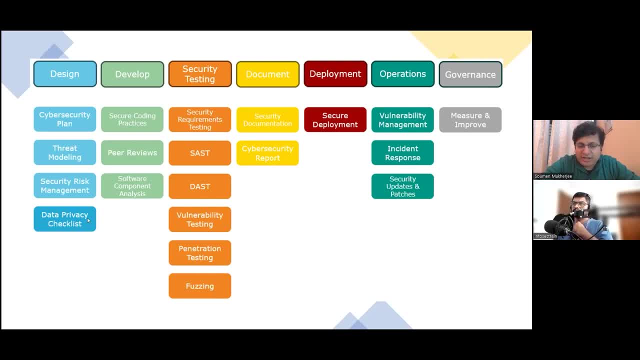 of your design. it's not. it is not an afterthought, so it is also something that i personally recommend: that, yeah, you should consider it as part of your design phase itself. so this is again something that is happening, uh, in collaboration with your first line and your second line. so 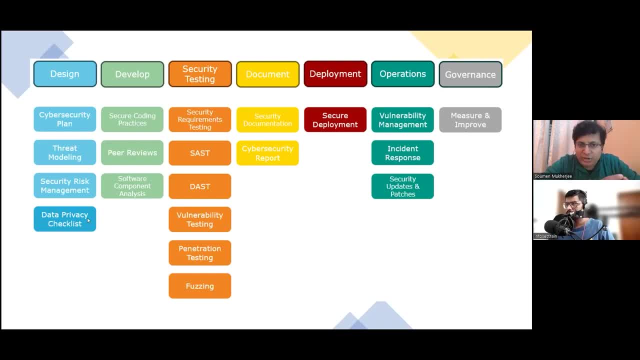 you can do that as well- of defense. so both have to work together in in this scheme of things, now your crm software development has started and, as i mentioned that you have encode, they are raising prs, it is getting reviewed, it is getting committed. so that is where your secular coding 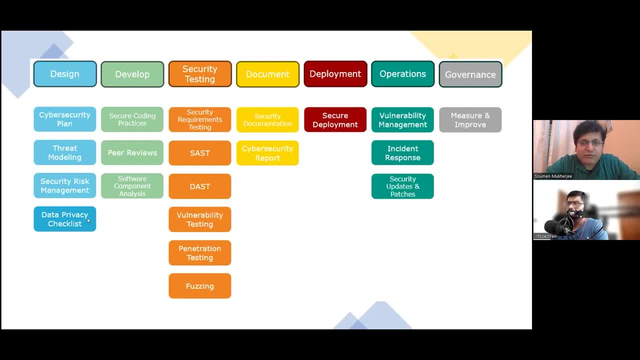 practices comes into play where developers have to basically follow some kind of a guideline, or they can also use some automatic tool because see, you know, these days there are being such a dynamic uh thing, you know, it is really not possible always to people, for people to be really up on speed with the secure. 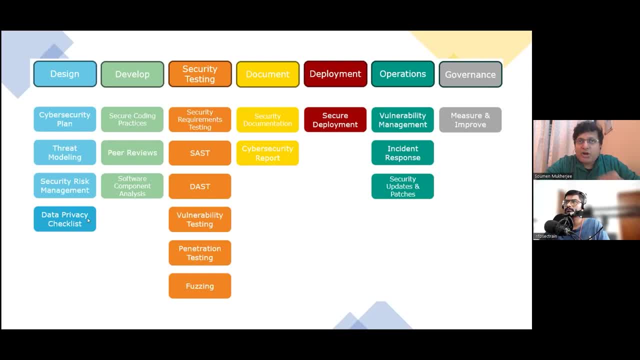 coding practices and with the guidelines. so, in order to mitigate that gap or mitigate that risk, we can use, uh, our tools which which help us to write secure code, and then those are the tools that we use in order to make sure that we are really engaging the users. 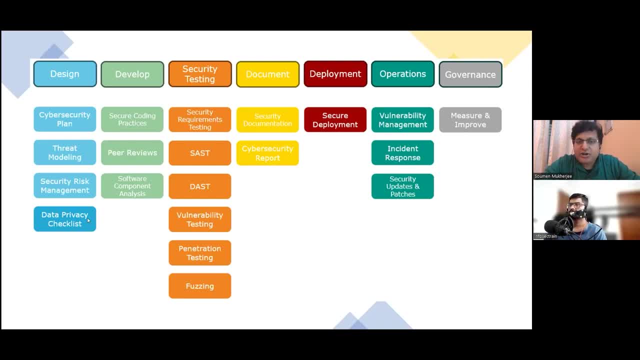 so i'm going to flip this over here so you can see here, you can see that, uh, the code has been updated. so you can see the code has been updated. so if you want to update your uh code, it has to be updated. um, but i haven't seen it yet in a few months. so this is what i believe and like to say. 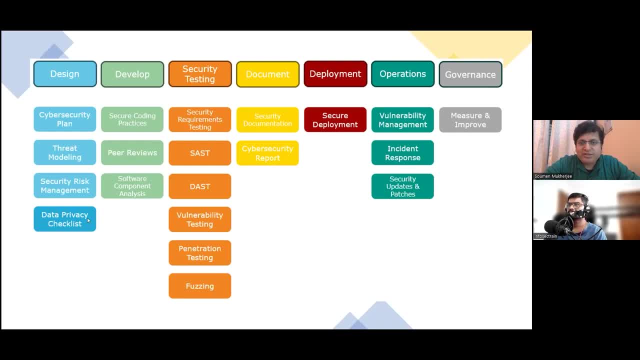 this is an excellent idea, so it is a good idea to come into the domain itself, because you can do so much better with your code. so i think the other thing i wanted to mention is the peer saying this code is fine, but the security architect is saying that i should not use this api. 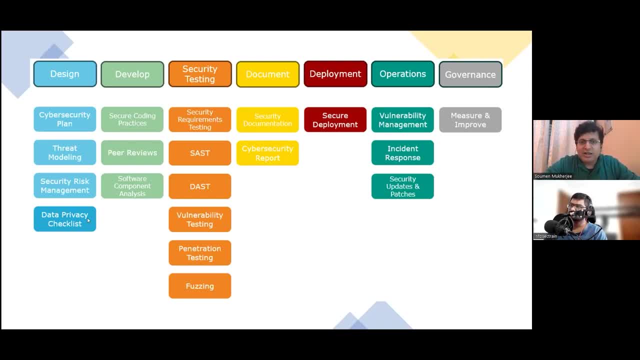 or i should not use it in this manner. and that is where you know then the security architect and has to use his convincing abilities, in his skills, to explain the situation, the best practice, and then you know, things move forward. another dimension here: uh, in the part of the development which is 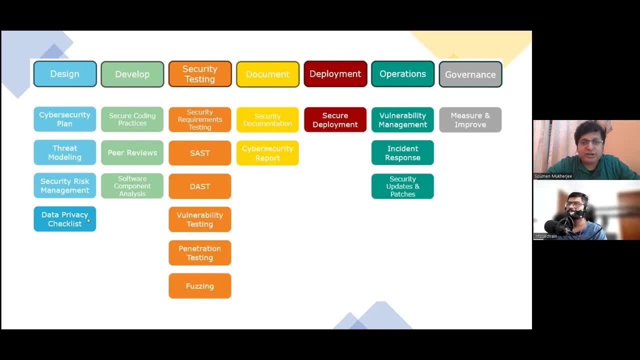 now becoming very popular is uh, the component analysis, or software composition analysis. essentially because, uh, for people who work exclusive or, you know, extensively in the us industry with federal customers as form has is now a mandate. so what is this seo all about? like you know, i have there's a lot of buzzword around this sc. i know you told about federal mode, so those who 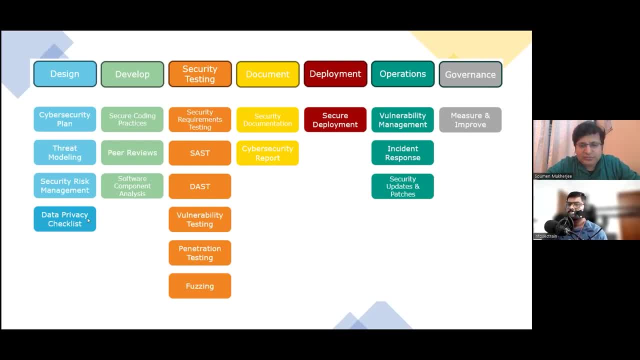 so i'm sure some folks who preparing for cs, sp or cc, spc, sslp- this topic is very buzzword so and i've seen a lot of people get the question interview questions asked on this area. so is it possible for you to spend two minutes on the sca? 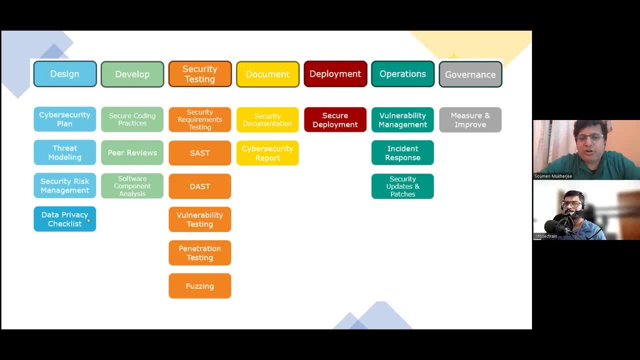 yes, yes, sure, sure, sure. so basically, when you talk about software component analysis, so we should actually first try to understand what is bill of materials. so people who are- uh, maybe who come from a hardware background, or who have worked in a production line, manufacturing line for them, it 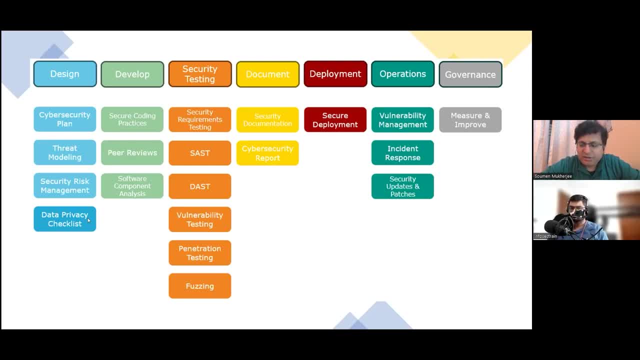 can be that way: if you are a builder, that you have a lot of experience with the material, you are able to sort of learn from those examples. so if you just take an example of, uh, let's say, this glass that i'm wearing, so it has a bill of material, what it's built of material is bill of. 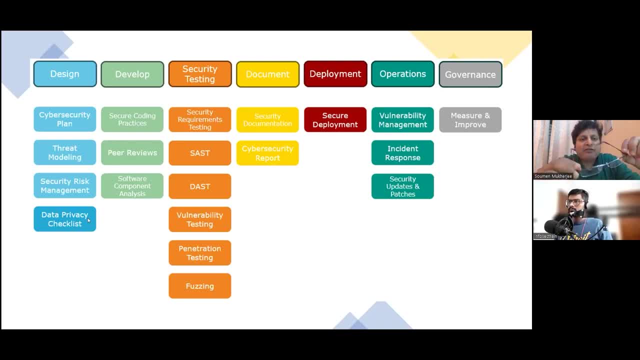 material is all the list of sub components which are used to assemble this end product. so it will have a, let's say, a frame. it will have a couple of screws. yes, it will have the glasses. it, when you put the list together, uh, you can say that, okay, glasses, you click on on a, on a button. 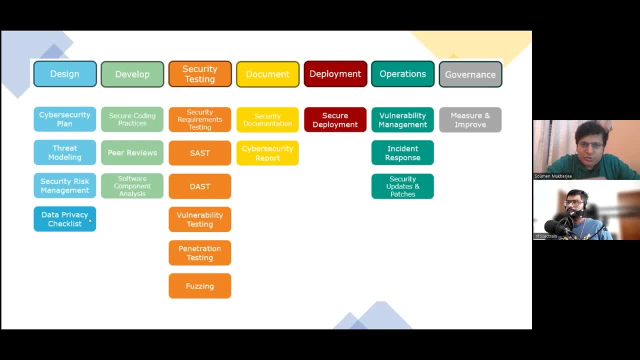 and it lists out the bill of material. it will have, okay, screws, frames, glasses, pads, color polish packaging material, everything. so that is like a typical hardware bill of material. now the same concept has been ported into the software industry and that is what what people say: oh, let's create. 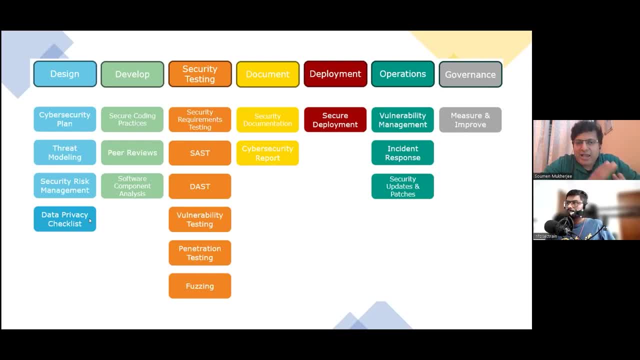 the s-form or the software bill of material for any software, any service, and that is basically. it then comes under the software component or composition analysis where we say that, okay, what constitutes the software? you know today, no software is, uh, written from the scratch. there are a lot of packages, almost every software you know. 60 to 65 percent of it comprises frame. 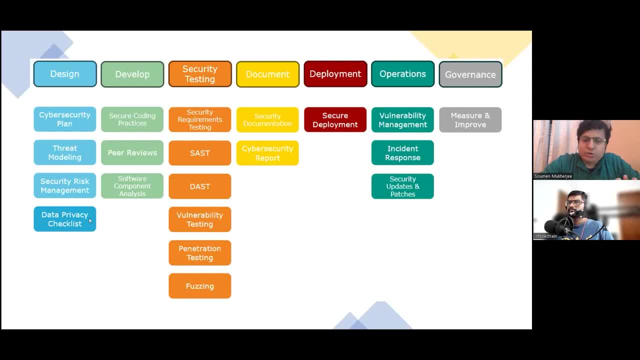 works libraries packages. some are open source, some are licensed, some are redeveloped by other teams within the organization. so you know, so it's a composition, it's something that you basically put all together and you create a software, and that is where the s-form comes into picture. so s-form 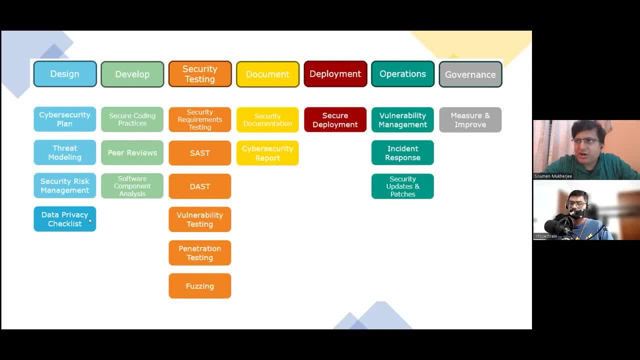 basically, it's a representation of the composition of your software. there are various formats which are popular, like one is spdx and then the other one is the cyclone dx. cyclone dx is something which is open, uh, more popular because it's uh supported by ovasp and us federal agencies. uh, basically, they. 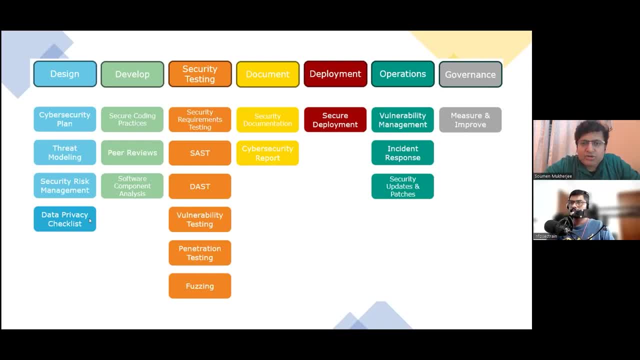 accept spdx as well as cyclone dx format. okay, so in a way they are like json files, but then there are a lot of different attributes which are defined within an s-form. interesting to know for people who are new to the concept of s-form: that s-form 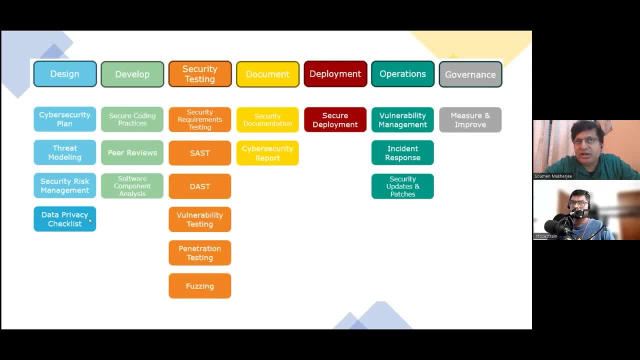 uh, not only has the uh, as per the definition, not only it can basically tell you about the components or the constituents, it can also tell you about the vulnerabilities which exist in those packages. so the format is very extensive and uh, it basically gives you, uh, a list of vulnerabilities also which are present in the packages. so the 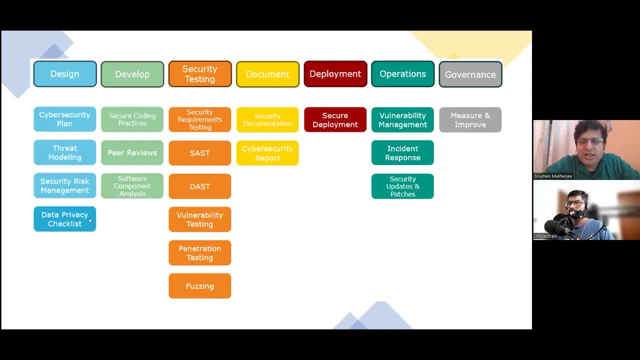 idea here with s-form is to bring out more transparency in in the software community and, uh, you know, this basically became more popular, or i would say the industry realized why s-forms are needed. when the log4j vulnerability was: uh, who, who will, who will? basically forget that. 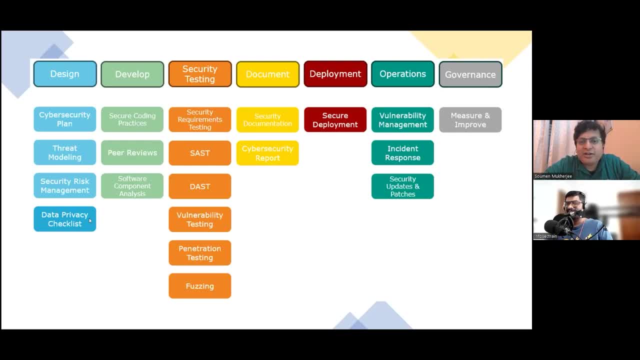 right, spoil the weekends and new year's. yes, it's spoiled the new years of people and that is when people realize we need something where we can say and we can go and say: okay, where all log4j has been used and this was a million dollar question and, trust me, for a small company. 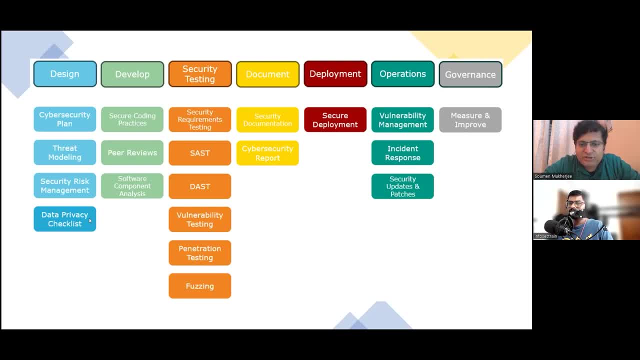 even like where i work. it took us a few days to basically outline and discover where all the log4j is used. and i can understand for larger organization, larger enterprises where there have been, you know, tons of services and software developed. it was a nightmare so typically. 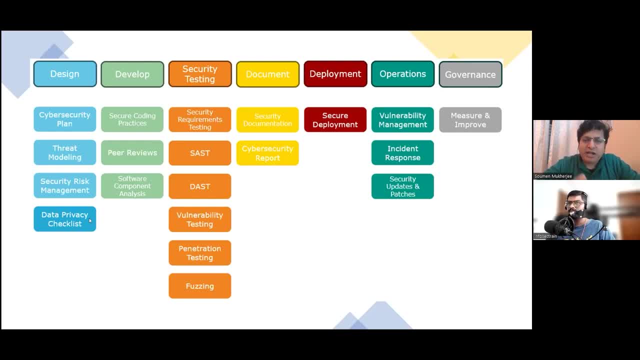 uh software composition analysis. when you maintain a repository of all the s-forms, you can do a search on a component and you will get to know where all this component and this particular s-form has been used. that is the real power of s-form generation. is the first step, the s-form 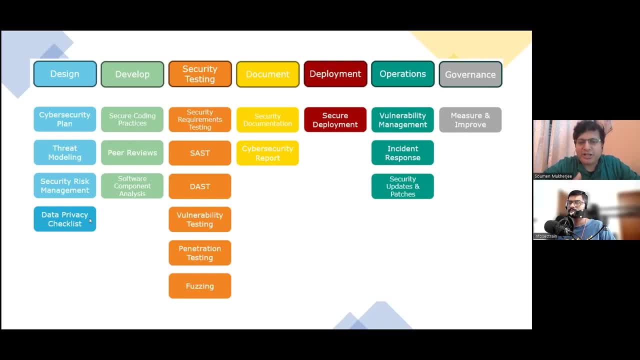 management is the next step, where it becomes really powerful. that's great. so you know you do all this as part of your development. and then, very interesting, or the very important part- now, as you develop your software, you also test. now in agile we have this continuous loop of 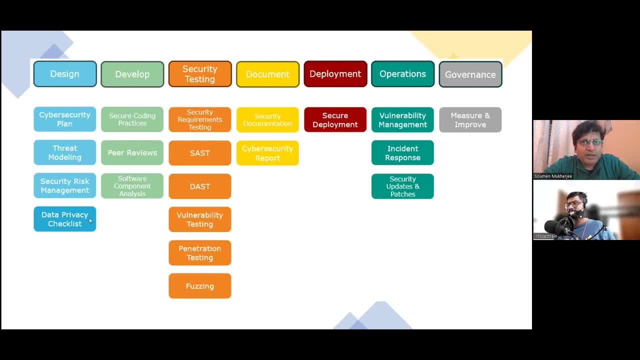 development and testing, and this is where now you see that you do all the security testing also as part of your software testing. and you you will notice in my diagram that the left side is heavier than the right side, right. so what it means that you do more stuff in the beginning than you do to save cost and time. 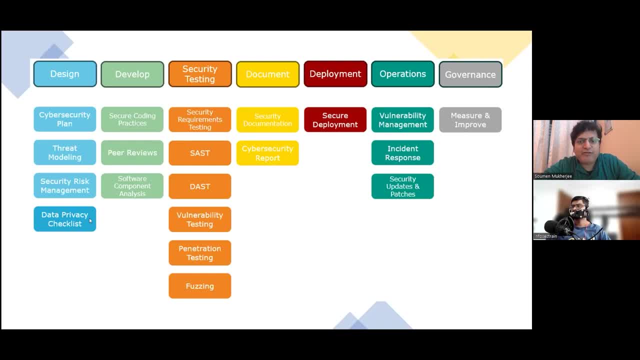 right. so this is what essentially is the shift left paradigm, where you basically shift your processes, your security processes, to the earliest phase of your development, because that is where it is cheaper for you to address issues, to fix things, and rather than doing it the later stage. but i want to say one thing, dada, here: this part of the content, what you covered, it was an eye. 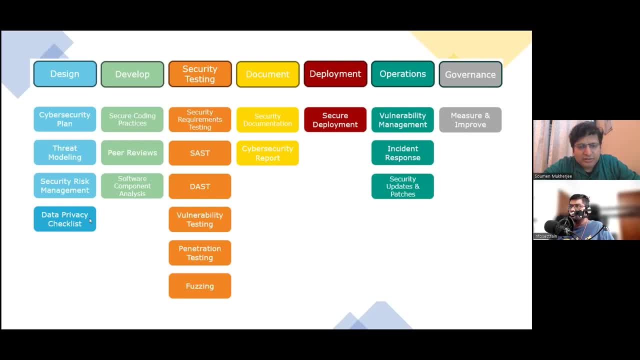 opener for me, to be frank, and i haven't seen any video which talk about so detailed about the sdlc from this perspective. thank you, dada. yes, no, no, this is very important. this is the. this is typically you talk about. you know, i don't see a lot of security architects in the industry. 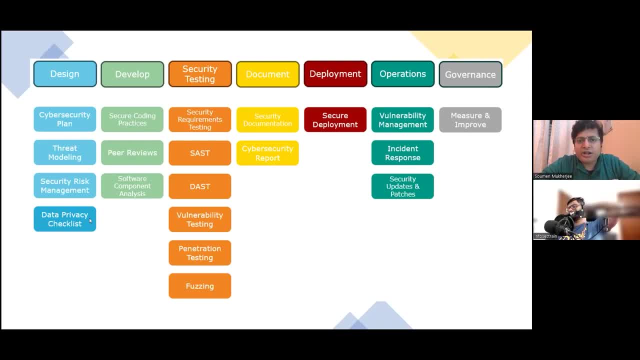 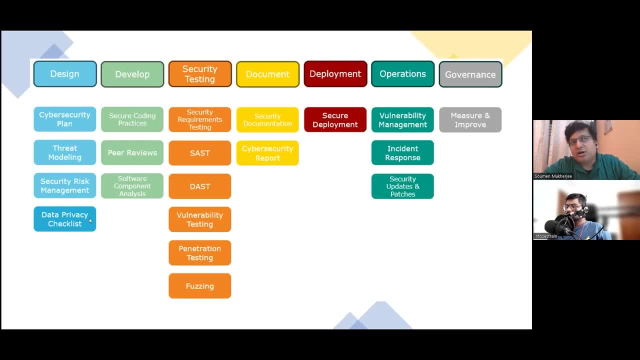 because of the vulnerabilities that they actually cause their users to actually suffer damage. right, And this is what we would like to avoid by having a secure development lifecycle, And this is what it is trying to address. Great, So you talk about security testing. 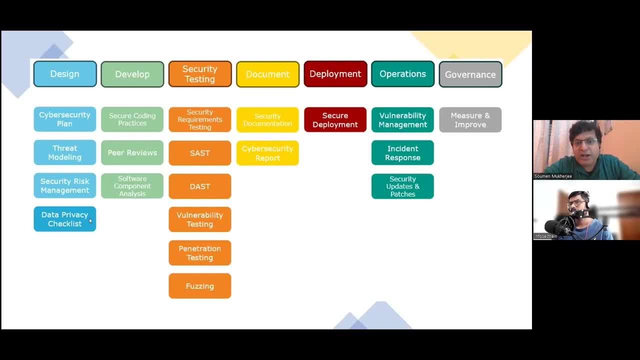 You have security requirement testing. Now, very interesting concept. I would like to point out that many people basically say that, okay, let's try to. you know they say that. okay, we have a user login mechanism. We have a password change feature. 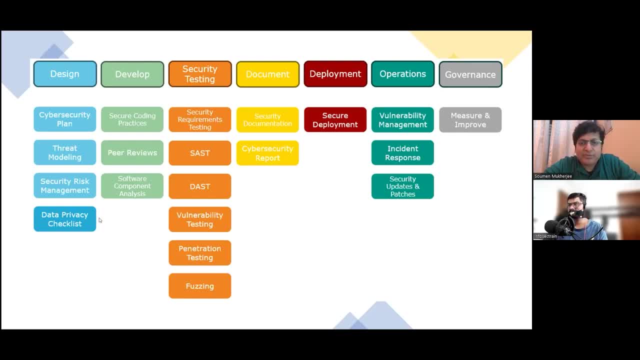 We have, you know, a password reset feature and all that. They basically consider it as part of the functionality. But I look at it differently. I say these are security requirements. Yes, So you need to have a clear distinction between your functional and the security, you know, requirements. 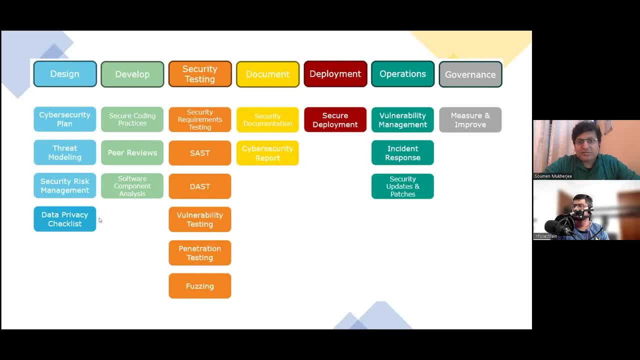 Because security is considered as a non-functional requirement. correct me if I'm wrong. Right It is. But you know some people they say: well, I have a functional test plan. I'm covering my change password login test. 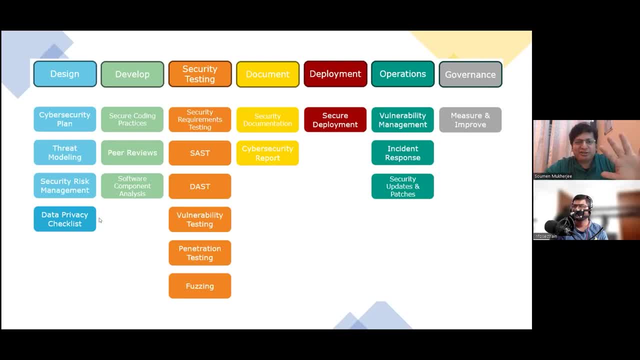 But that is just five test cases you are doing right. But that is not covering your security of your password reset flow, right. It is not covering The security of your user login process. It is not covering your user login experience as well. 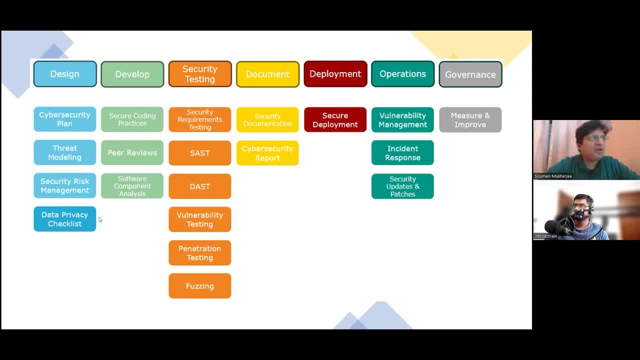 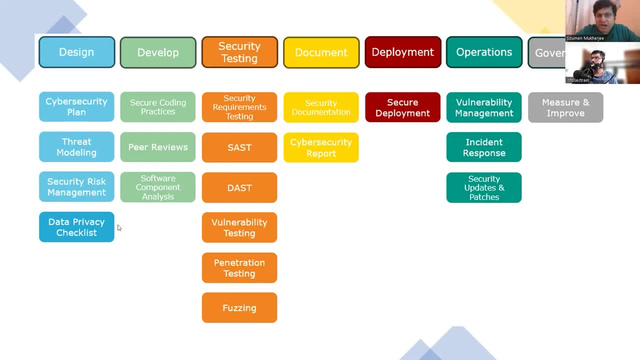 So that is just five test cases, So let us not talk about it. So let us talk about security requirement testing, Right? So to me, you need, depending on how important or how critical the product is, you need to have a security test plan. 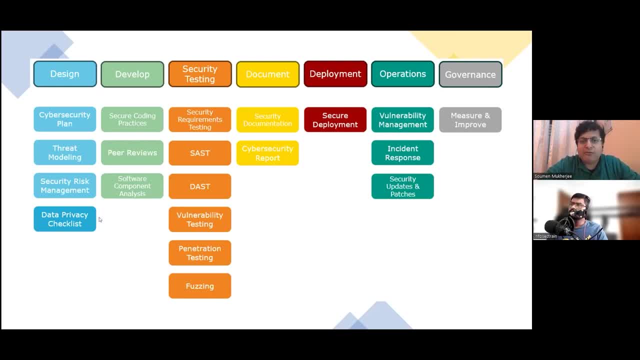 That is what I say. Where is your security test plan? How are you going to test your security? What are the tools that you are going to use? And that is where the other steps comes in. What is how? what are you doing for your software? static analysis. 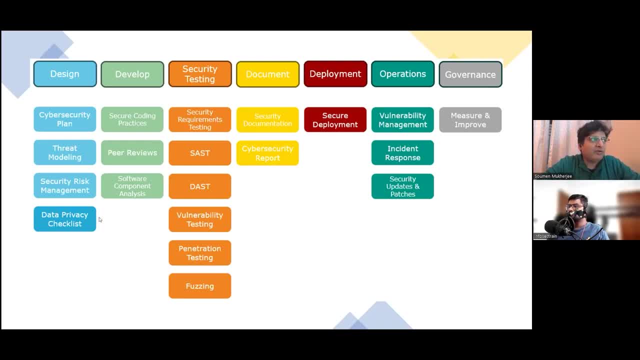 What are you doing for your dynamic application security testing? What are what are you doing for your vulnerability testing? Is pen testing part of your scope or not? Are you doing fuzzing for your APIs? Because that is where you know now, there is no system without API. 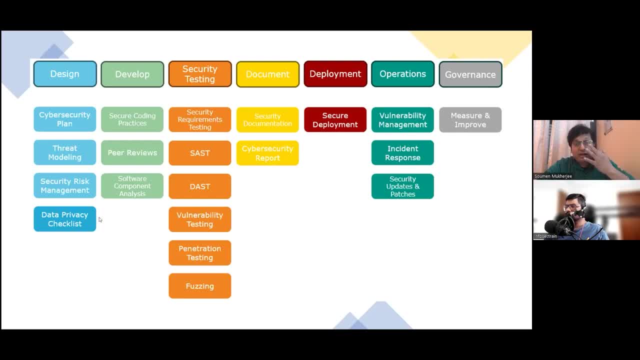 So you know you need to, You need to have fuzzing, You need to have that ability where you can really create that kind of a situation for APIs where they, you know, basically lose their normal flow of operations and they start behaving in an erratic manner. 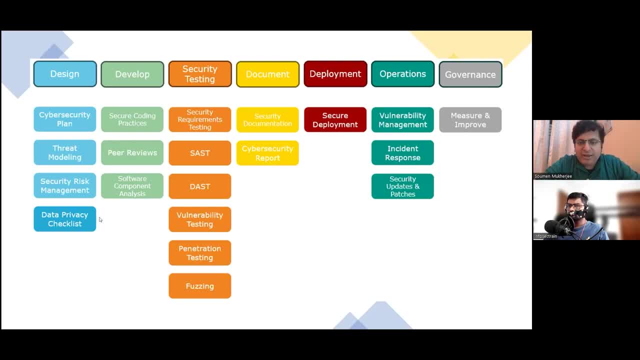 And that is where you know that. okay, if my APIs are now out of control, is my product secure? Is it? is it maintaining the three triads of security, which is good? Markoz Januc, port and file security of actually têm no Tamam. 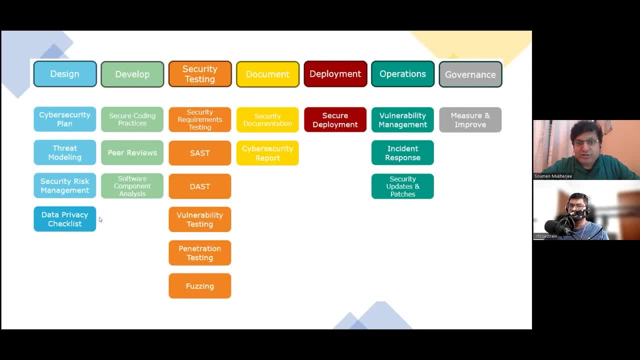 That is how you might access Fidenciality, Integrity and Availability are my three pillars intact. So all you think you do Software application static implications security is. testing is a is a domain in itself. You know we can talk hours about AST application security testing. 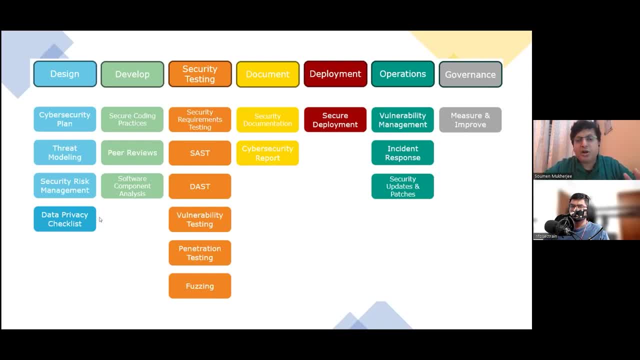 There is. there is a separate magic quadrant For AST. God does you know? That is how important It is. still don't have AST in place. you know? DAST again, there are numerous ways you can do DAST. but yes, very popular burp suit, people use it extensively. good, I'm very happy, I feel. 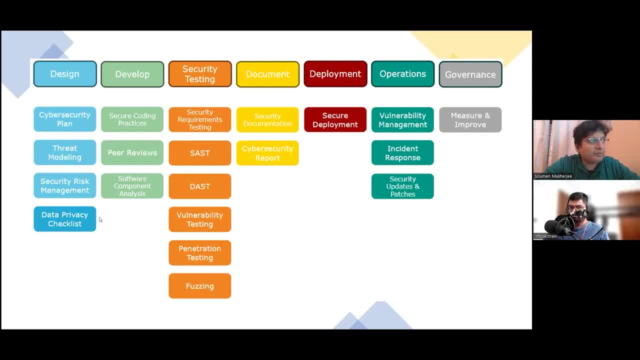 very happy when people say, okay, we have done a testing through burp suit, but then is it structured? is it? is there a process? is it this is done with a method? is it done with the objective in mind? you know then, but does here what? when you talk about the security, 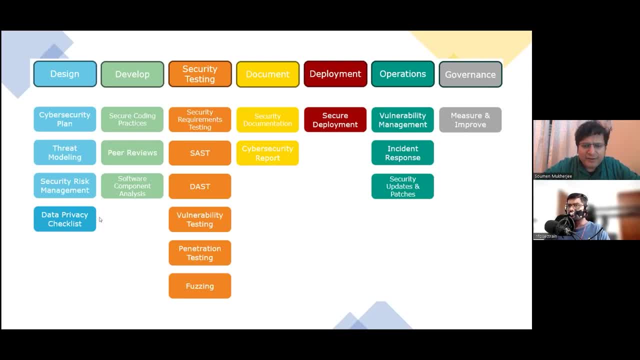 requirement and all that. do we maintain any kind of a documentation like what I heard about? when you're talking about documenting requirement, we have one factor called security traceability matrix or requirement traceability matrix and all this. so do we maintain such kind of a document or? 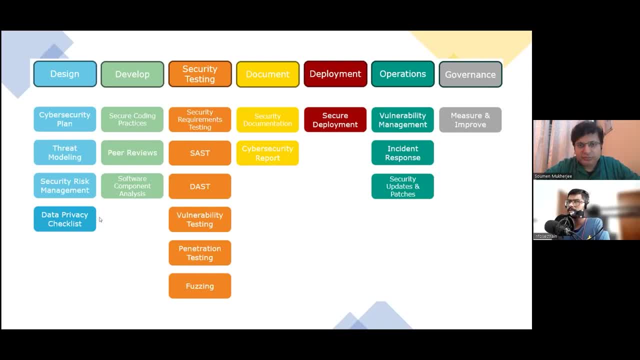 what exactly we maintain how, how are we organizing the security requirement testing, right, right. so typically, what I've, what I do and what I also recommend people is, of course, and let us be practical also, like everything cannot happen on day zero, right, it has, it has, it takes some time. 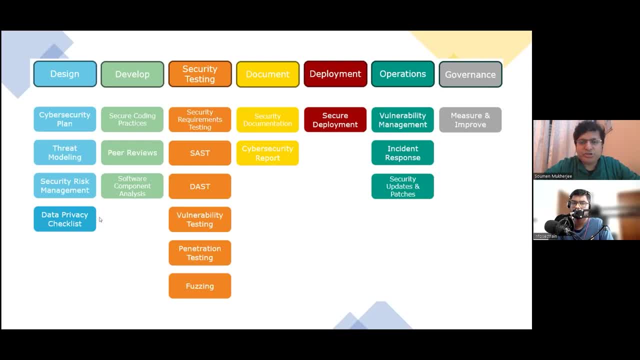 you know, because the resources are limited, even organizations, they will say that, oh, I cannot invest this much in security. I can only invest this much. so we basically take a risk-based approach and say that this is how, this is what we will do first and this is how we will scale up things. so 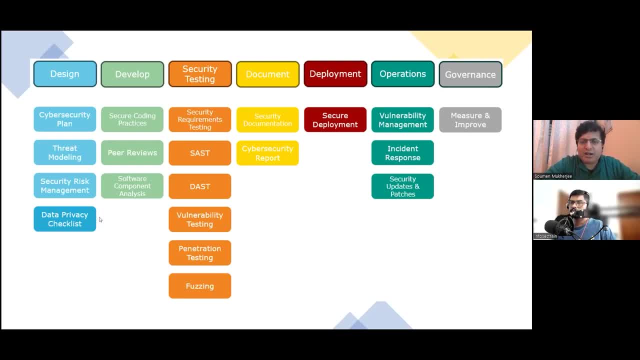 typically what we can do is we can have a security maturity matrix where we say: where we keep a record of, when we keep a measurement of our security practices, that, okay, are we doing fast, yes, no. okay, if you are doing yes, are we doing it in all branches or we are doing it in some? 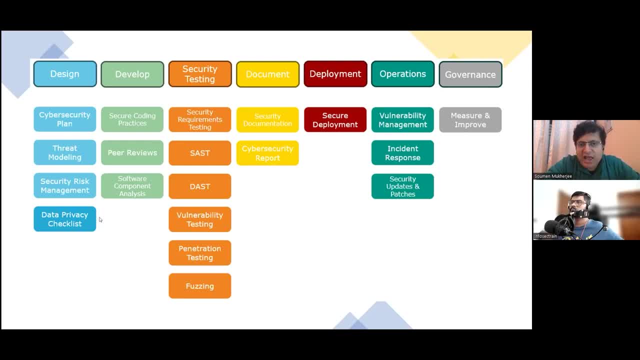 or we are doing, just doing it in on the master branch, so we can have a security maturity matrix. so if you look at the last step, which is governance, which talks about measure and improve, so that is basically if you start measuring your maturity of your security practices. 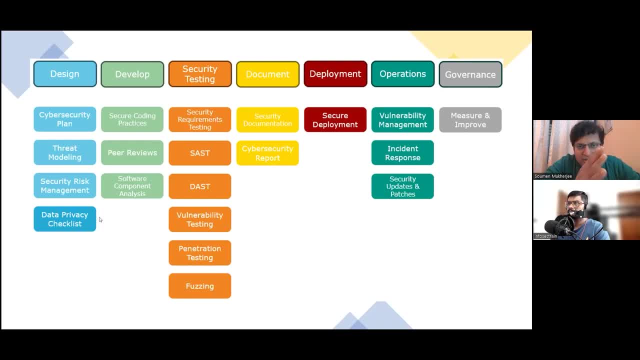 you will get metrics for your KPIs and also for improvements. that okay. today my level is this: I am doing it on an ad hoc basis, but I would like to improve where it is done as part of every release or it is integrated with my CI CD pipeline, where my build once it 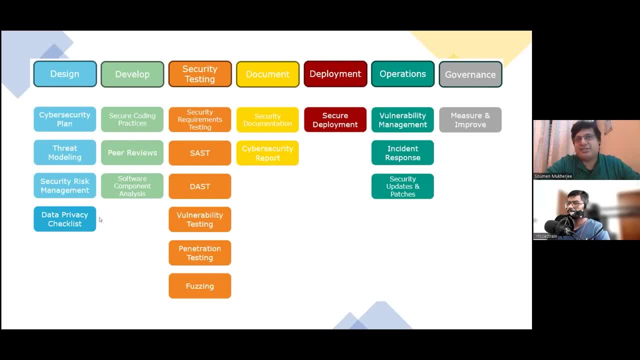 is deployed. it is also. it also initiates a DAST scan from from the tool that I use and you know the report is generated and it is emailed to all the stakeholders. so you basically have a security maturity matrix that you can use and that can help you to measure where you stand with. 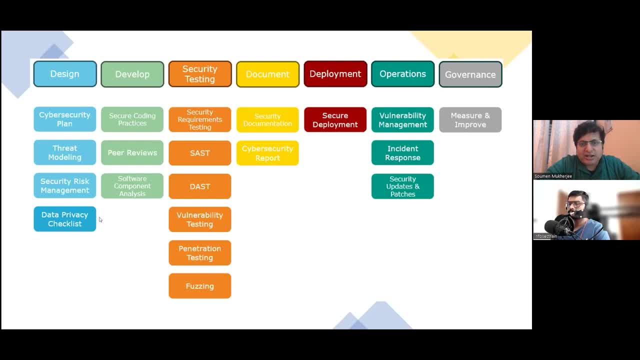 respect to your security practices and it can give you that nose numbers. where you can, you can use them further for improvement. right, so that is how essentially now you proceed. you basically also document. you do your security documentation typically. uh, now I see that a lot of products they also come with their security hardening guide. 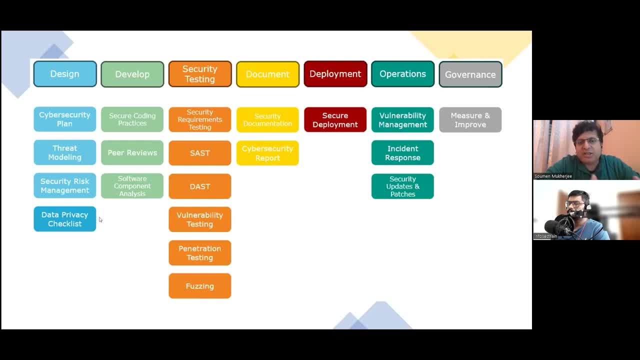 you know that, okay, this is our basic configuration, but this is a hardening guide where you follow these steps and you basically turn off services which are not required, or you know, you make it more robust, more resilient against external attacks, and you also have a lot of videos, like Xeon, where you can get a more secure experience. the next step is: 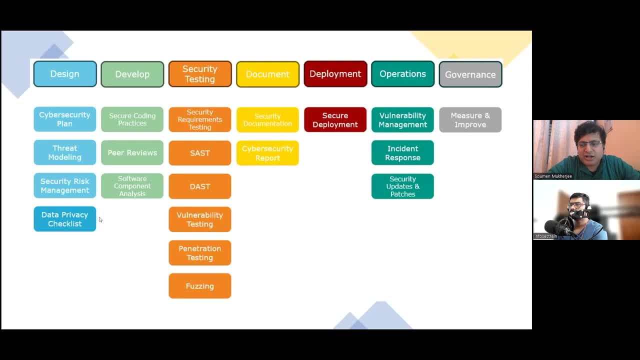 what Social Security does. it's a lot of security tools. you know. we see a lot of things like Code Connect, which is a lot of things like security, site security. and then we also see many times you see- security white papers where basically you talk about at a high level. 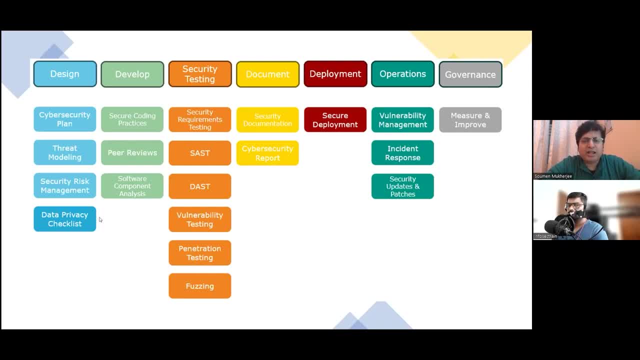 what are the security features or security functionalities that are available, technical and security stuff which gives a pretty good uh foothold to also to your sales people. so if you as coming back to your example of crm, so if you take when you the product is developed and 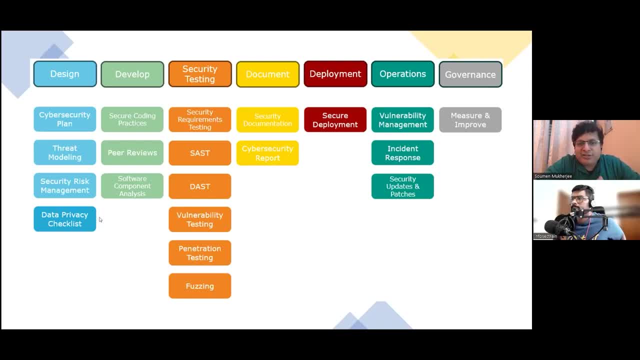 when it it goes to the market, you know most of the it guys will say, okay, do you have a security white paper for your product? can i have that? can i get a first-hand visibility on what? how secure is your product? you know, that is, i think, the first thing. uh, any it team will do. 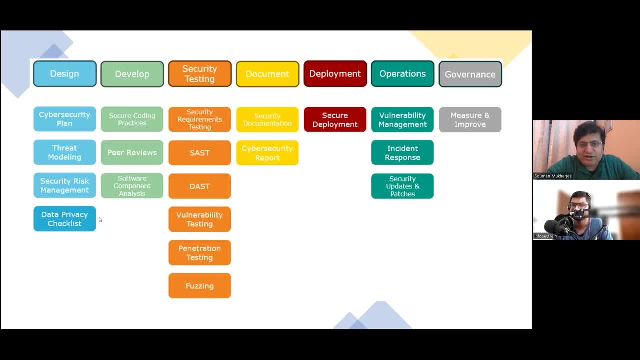 when they get a product. uh, you know reference from somebody from the business. oh, okay, this looks good, this is functional. can you look at the security part and they will ask for the security white paper. um then, uh, cyber security report. typically, again, it is part of the pen testing. 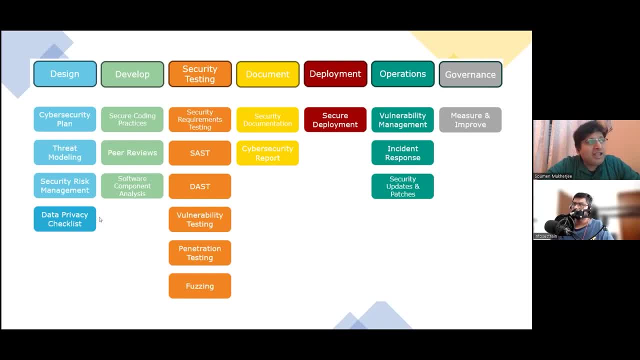 process. uh so generally, uh, pen testing is an expensive activity. uh so, and again, not many organizations maintain a pen testing team in-house. there are various reasons for it. it is more to do with the independence and the credibility of the pen testing reports, so that is why it is always. 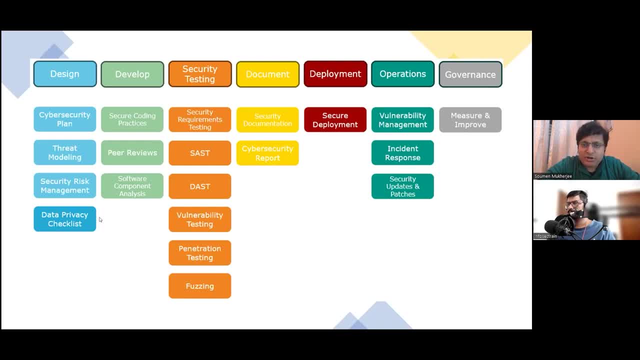 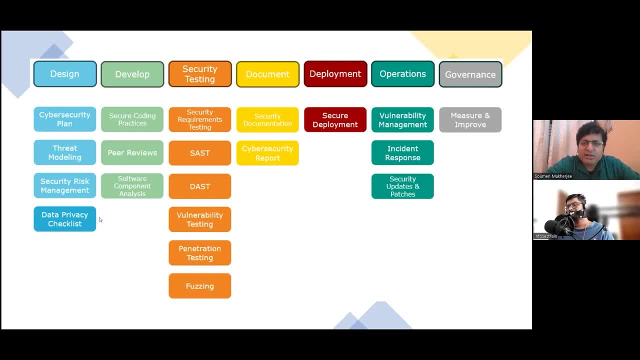 hacker will try to approach your system with very minimal information about your, the internals of your system. true, so you know you have to have that cyber security report. uh, now deployment again. uh, typically for sas solutions, this becomes very important that when you deploy your solution, your configurations are secure, right. so. so typically, you have to have a review done of. 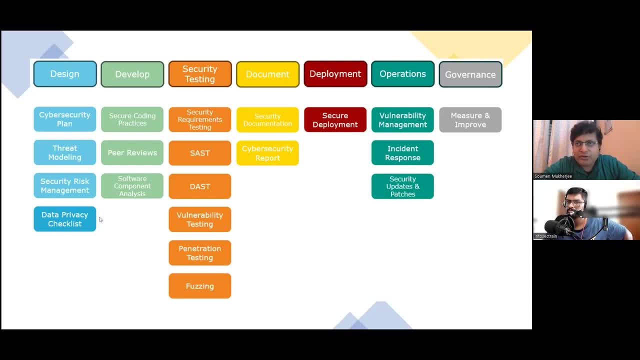 your deployment strategy, your deployment model, your deployment configurations and- uh, that is where your secure deployment becomes very important. okay, now the interesting thing comes. that deployment is done, product is up and running. now people will say: ah, security is over security. sorry, it has just started now. now you are in business, people are using it. now you will 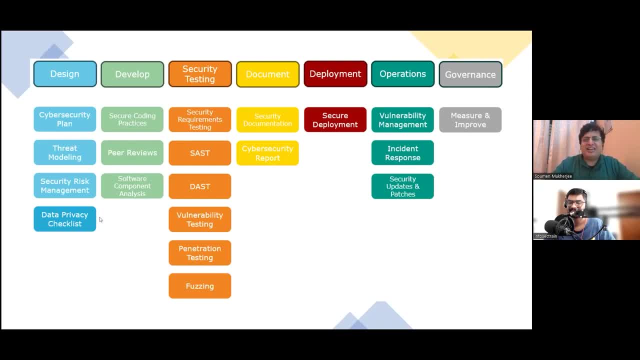 attract hackers. now you will attract attention. so till the time chat gpt was being developed, nobody was really worried about what is the security and the privacy matters. the moment it went online and people started using it, suddenly people realized: oh, what about security? what about the information disclosure? what about my privacy? what is happening now? it is the your operation. 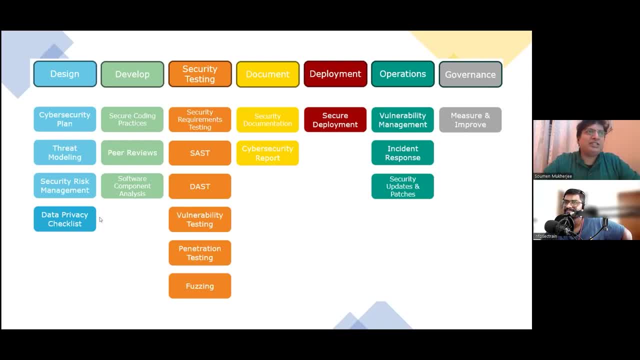 starts. that is where you have to now become extra vigilant. you have to. you have to be ready for any security incidents. right, you have to be ready with a response plan. you have to be ready with a security incident response team. you know that. what is supposed to be done? let's say the system. 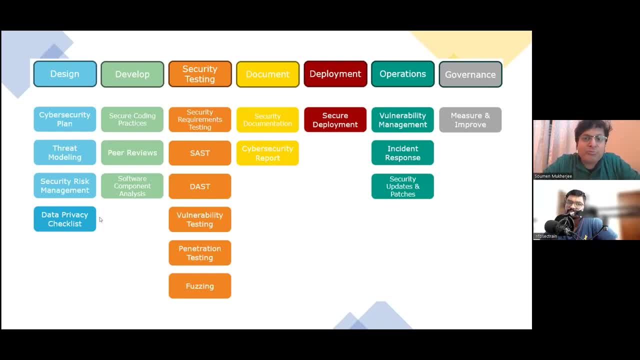 gets breached, what has to happen, what has to be the flow, who who are, who is going to be in charge, who is going to be in the driving seat? so incident response is very important. it's some topic i think you will also agree from that. again, we can talk weeks about incident response and we will still 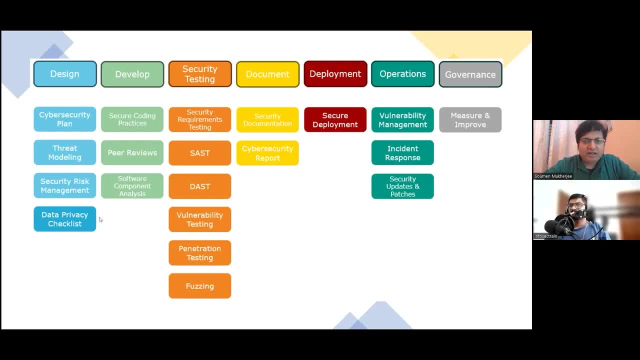 not be, you know, through thorough with that. again, that is the kind of topic. it is right, there are various compliance things which are associated with incident response. you talk about the upcoming regulations in india. you know security incident response is going to be very important even in the indian context so far. occasionally we keep hearing news that some data 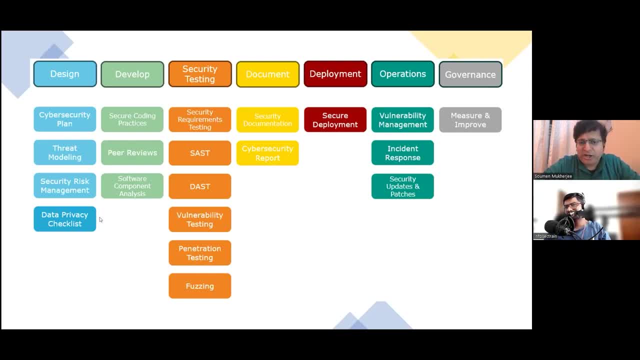 is available in dark webs from some bank, from some mobile operator people. they so far the organizations, have no legal bounding to come clean out of it. but with the regulations in place, it will be very important for the security incident response to be very important, for the security incident response to be very important. it will become important, it will become a requirement. 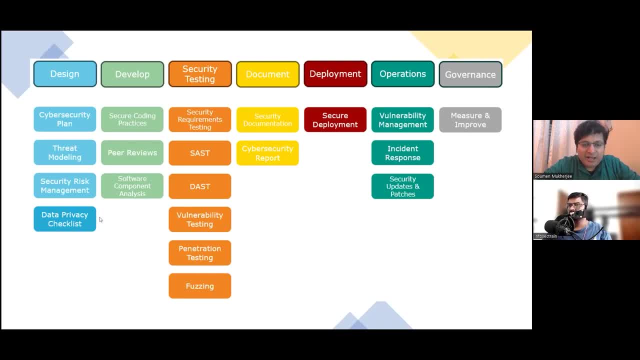 for them to have a incident response plan in place. so- and it is not something that is that happens in isolation, it is, it has to be part of your software development process, it has to be part of your software release process that, whenever are you making the release, is your incident response team. 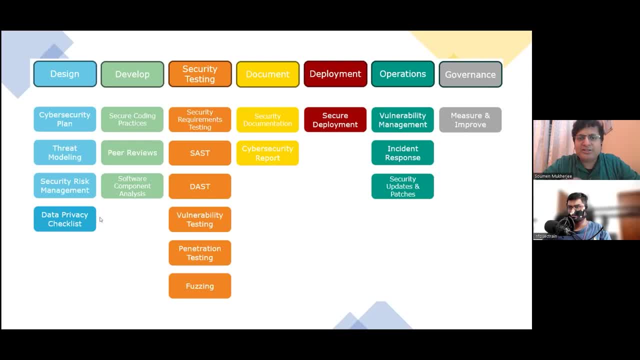 is it aware about the changes that are going to happen? is it aware of the new endpoints that are going to be exposed? is it aware of the new security controls or any changes, any breaking change that may happen? you know like typically people say that okay, we will change the password policy from the next release. we will 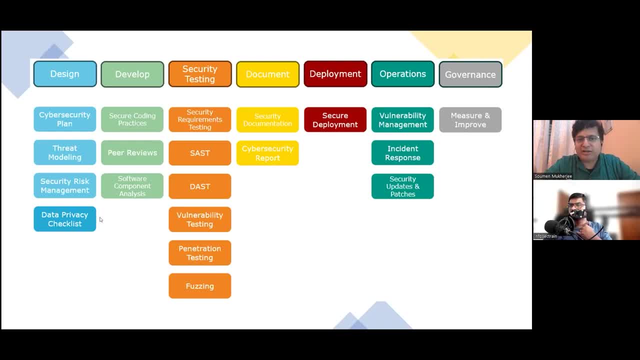 make the length go from 8 to 12 characters. so people will be prompted when they log in that you need to change your password. but in an enterprise, when the user comes in, if he sees that window- typically for a senior person- he will call the it. what is happening? it is asking me to change the password. i have you changed anything? 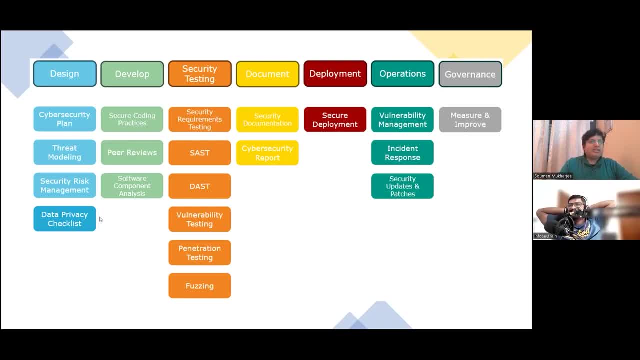 that would be the first question. so you know, these are practical scenarios. we come across situations just like this and these things are not really given that kind of thought or that kind of importance. and security updates and man vulnerability management i think very important. you know, this is the kind of mouse game. 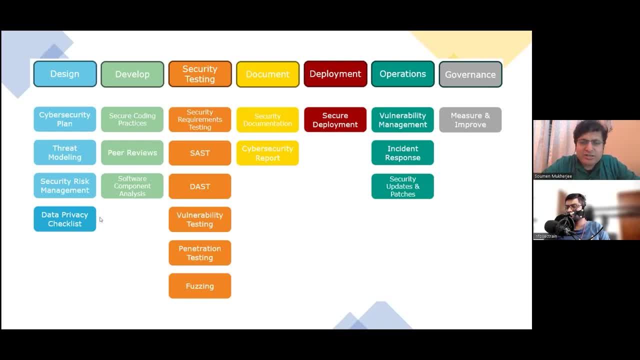 vulnerability will come, always come, in your packages, in your open source libraries. you will have to up your game there. you have to make sure that you- you are, you have a productive plan to update the patches. you know, typically i see a lot of sales people come to me and say that 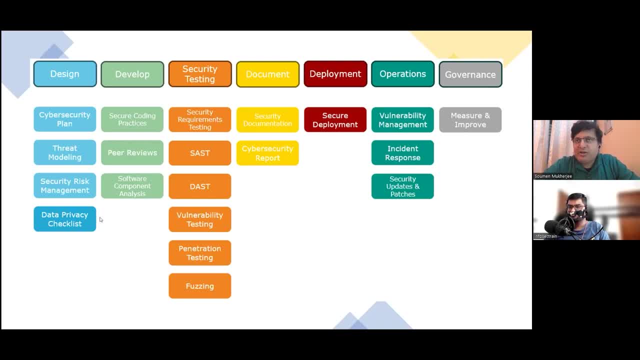 okay, how many days? in how many days we we do the patch, do can do? we do it in 48 hours, do we do it in 72 hours. so that is the kind of expectations that customers have and that is the kind of that the moment of vulnerability is declared in public. you patch it in 72 hours. you patch it in 48. 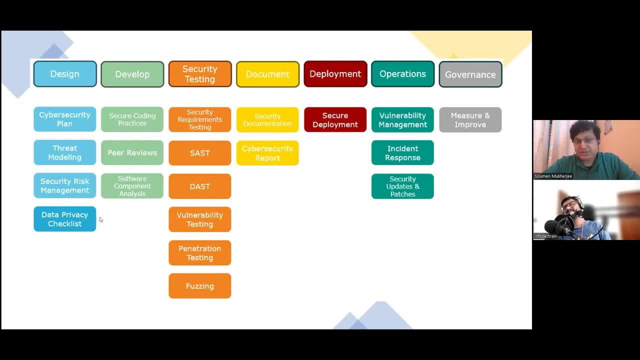 hours and sometimes it's a legal regulatory norms also right, yes, yes, in healthcare. in healthcare, yeah, you have to address situations in a matter of hours, you know so, yes, so you have to be ready. this has again has to do a lot with your security development life cycle. it is not an isolated thing. 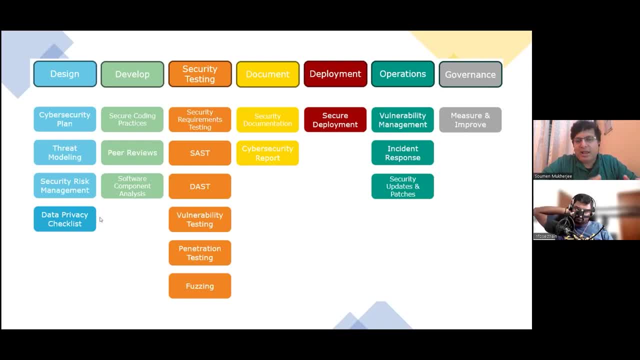 it has to be done in collaboration with the customer, so you have to be ready to do a lot with your R&D team and with your entire development team has to be aware of all this. now you take everything and now you say that, okay, i'm doing everything, but how can i improve? what is my 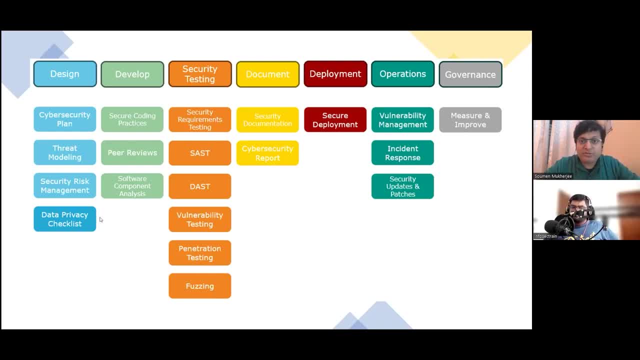 improvement for the next year. what is my measurement? what is my performance for this year? that is where the governance comes in and that is where you say okay, at the end of the day, i will measure. how many incidents have i received? how many high or critical incidents have i received? how many medium incidents have have i received? how much time have? 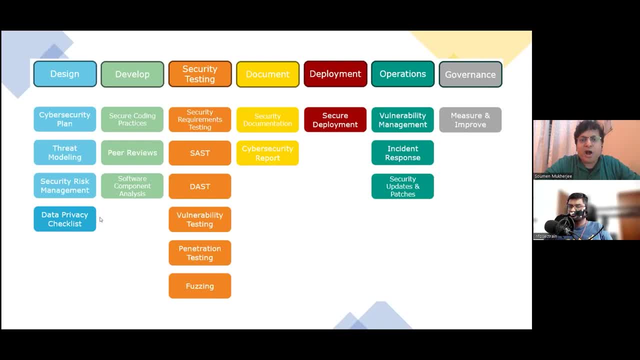 i taken to you know, fix those issues. what has been my? how many hot fixes have i given? how many security updates i have given? so you know all these kind of metrics. if you start collecting it over years, you know you will see that there is a trend right. and if you are, if you are really 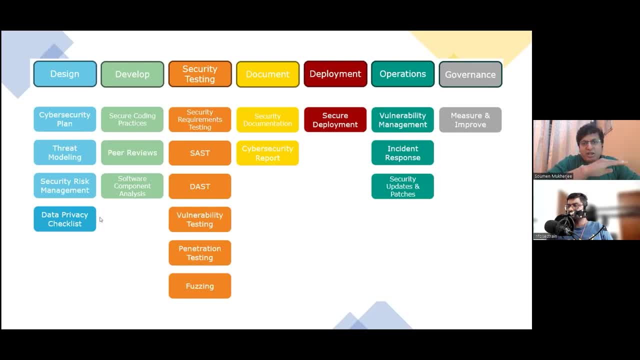 focusing. you will send that there is a, there is, it will not go down. it will not go down, it will always go up. but it will be a smooth curve right, because if it goes down that means you are not investigating deeper. you know the the level of disclosures have only gone up. if you look 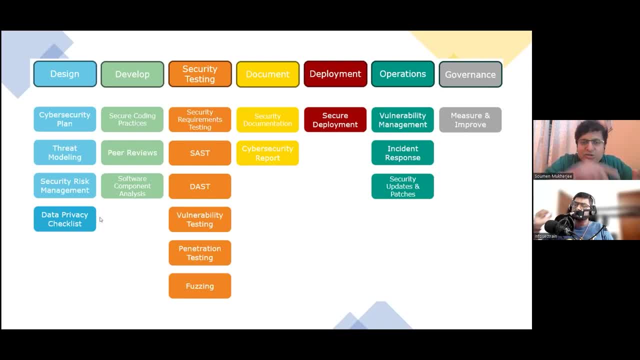 at the number of cves that have been released over years. so there is a. there is a exponential increase over the years. it has a direct relation with the software that you have written out, so you know. the same rate of increase should be there in the incidents in in your, on your site, because that means that you 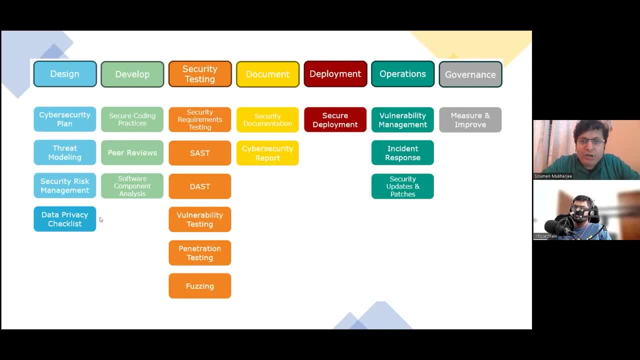 have been active, you have been detecting, you have been able to detect them, you know you have been able to address them right. so you know, you look at the all, all the things from the, from the software development perspective. from that you do everything and, uh, you know it's a. everything is related to 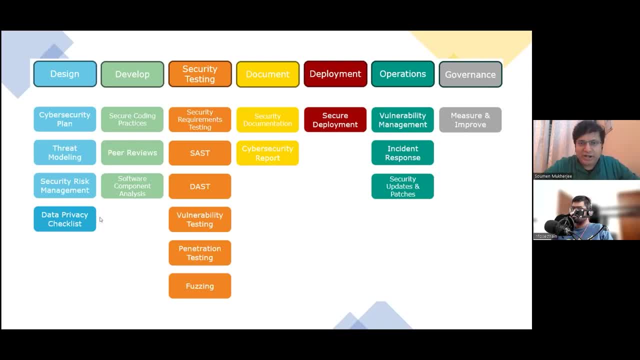 the previous thing and to the next thing. you know they are all interrelated. you can't say that, oh, i will not do documentation, i will only do security testing and deployment. no, it cannot be like that. you cannot say that, okay, i will do secure deployment, but i will not focus on operations. 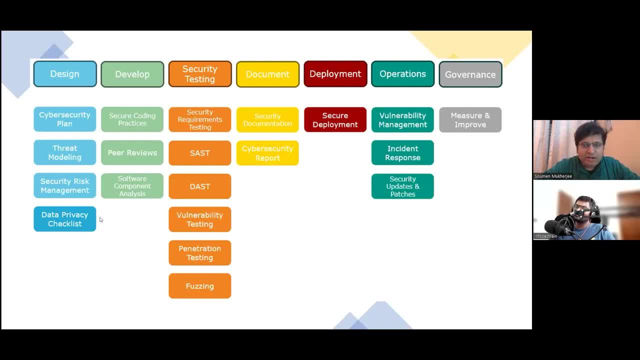 i will. so again, it cannot be. it cannot be like that. so it has to all everything has to be done in a manner where, uh, you know, they are all being done in a sequential fashion. so you know, that is, i would say, a very uh brief overview of of product security, product secure product development process. 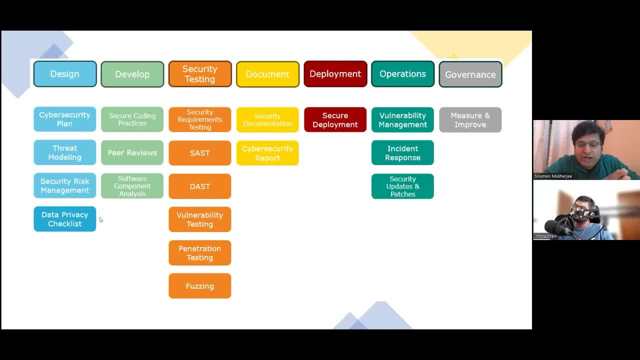 and how important it is for any organization to focus on product security, because it is not something that is only important at the time of being writing the software. it, it. it will come back when it goes for sales. it come, it will come back when it is being- uh, it is running in an operational 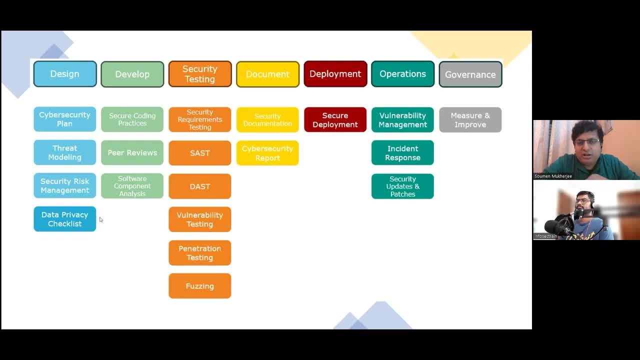 environment and it will come back when it is running in an operational environment. and it will come back when, whenever you know it, there is a vulnerability in the industry where people will start asking you questions and you know that is how it is. that is, that is. that is great actually. 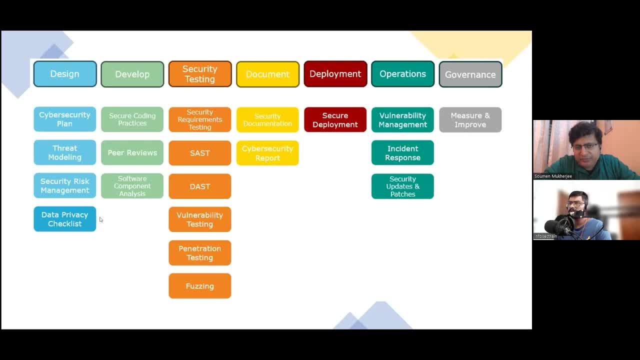 uh, so, like you know, you mentioned in the governance part, improve and measure. okay, so do you suggest any kpis which is can be very good for the sdlc, or product security? right, right, right. so one thing that i mentioned was, you know, measuring your product security maturity. basically you say that okay, again, that is. 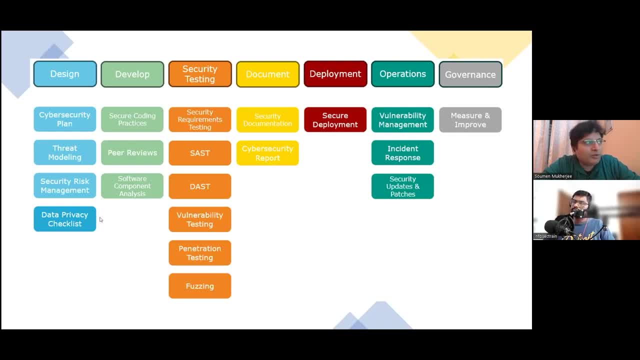 from from organization to organization. so you say that, okay, threat modeling, am i doing it for every feature or am i doing it for you know, for any major feature? similarly, uh, sast, do i use sast in in the all code repos or i do it only in the master branch, or 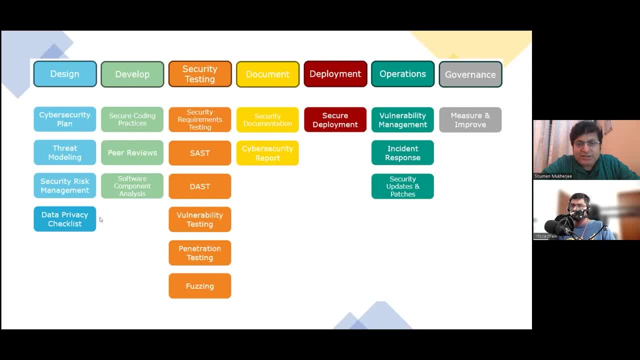 i do only in the integration branch- that. is it something which is ad hoc? is it something which is uh done, um you know, in a uh for every release, or is it something that is automated? similarly, penetration testing, again as i said that, uh, you know it's an expensive thing, so i cannot say i will do penetration testing twice in a year. 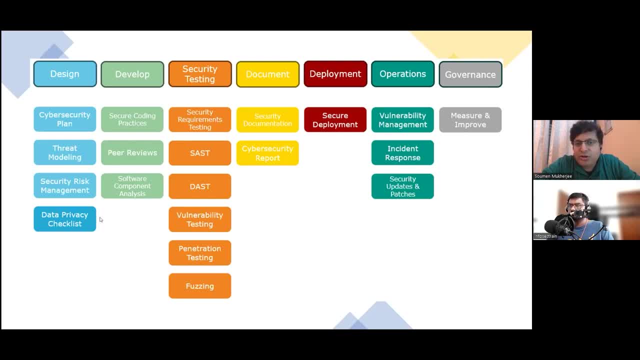 i cannot do that. i don't have that kind of money. so how do i optimize it? so again, uh, we have to be mindful of our time, effort and money. so we say that, okay, do. is it something that i do it every two years, or is it something that i do only on customer requests? so it again depends on the. 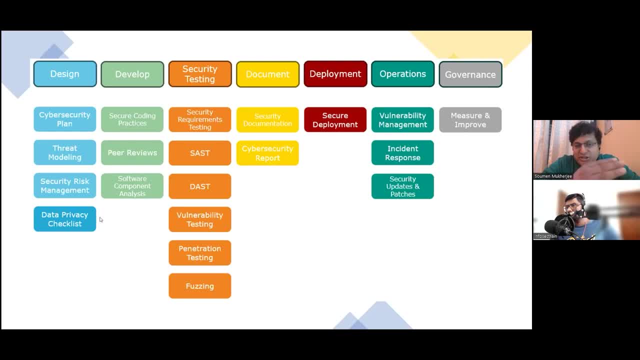 or you know, and that is how you start measuring it. so if you have this data for, let's say, two years, three years, you will then in a position to analyze that. you say, okay, i see that there is uh. uh, you know, the last part is something where the teams are lacking. and okay, what is the reason? 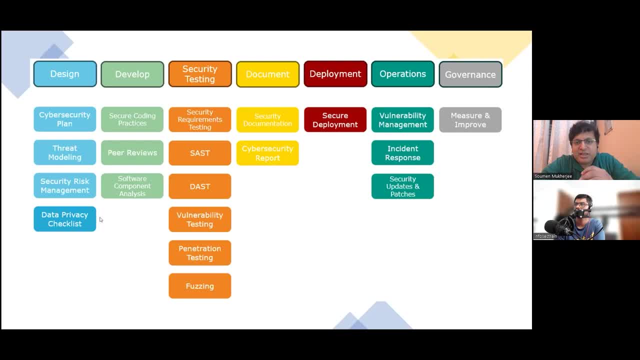 for it, why it is not being automated. people will come back to say, oh, we don't have that skills or, you know, the tool is not supporting automation. that is also a possibility. so with that kind of feedback the management can take, you know, improvement steps. that okay. 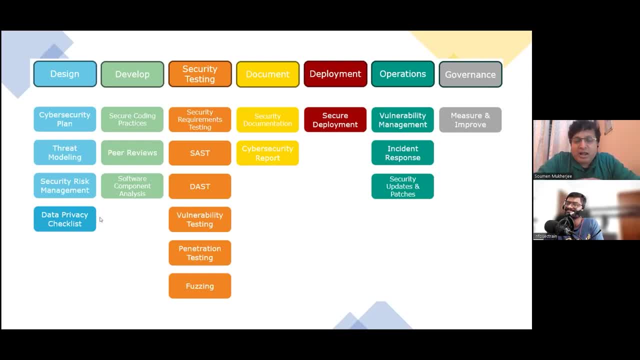 do we need to invent uh, invest in a new tool where it is something which is uh, which has easy integrations available with the devops pipeline, or uh, if the skill is an issue? do we nearly need to set up a separate uh dev, sec ops team that helps in the 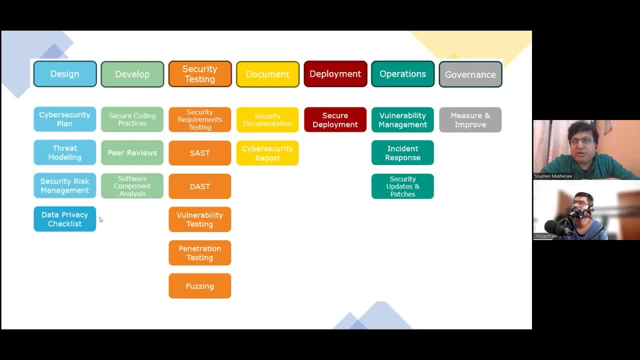 automation of all the things. so you know, such kind of measurement uh will give you those areas of improvement uh which you can then take up to the management and say, okay, because management will always ask for numbers. right, they will ask for numbers. you cannot say that my security has. 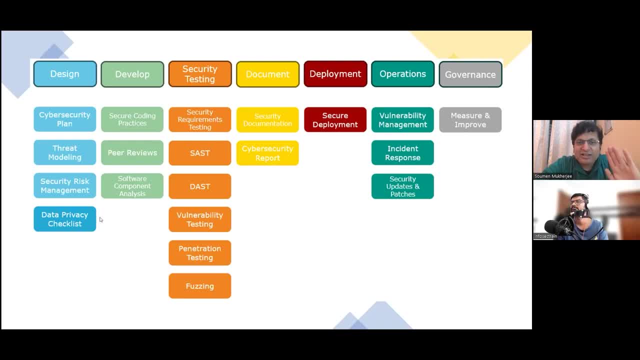 improved. they will say: prove it right, they will ask for proof and that is where you say the numbers. so okay, look at my process maturity, security process maturity in my there is has been an improvement. look at the security incident response: there has been no critical or no high. that has. 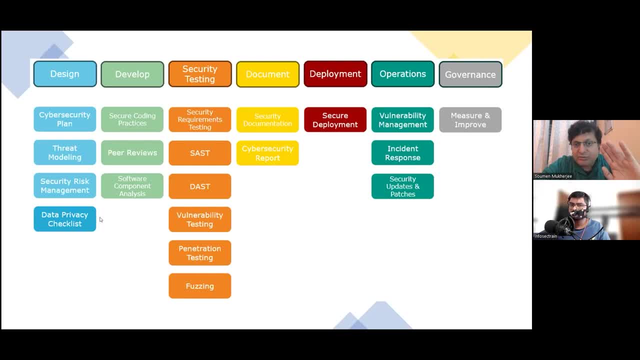 been reported. uh, from the field. you know, over the last two years, three years back there was one critical, one high. but now, two years, no critical, no high. so that means there is an improvement. look at my pen testing report. you know, two years ago these were the number of 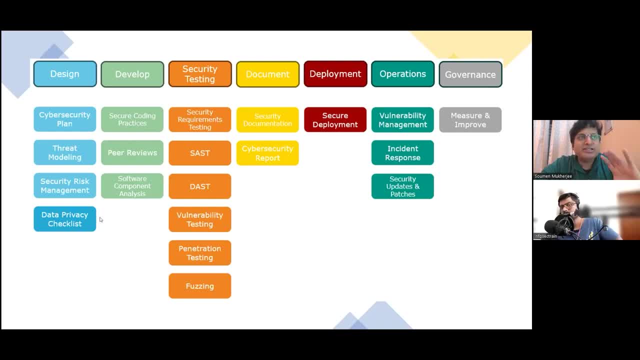 issues. now, these are the number of issues. so all these things will help you justify your improvement, your process, and it will basically be a vindication of the investment that the management has done in the product security. but that is a very good point. you have referred about, you know, the the maturity of the product, and i think we have a framework. 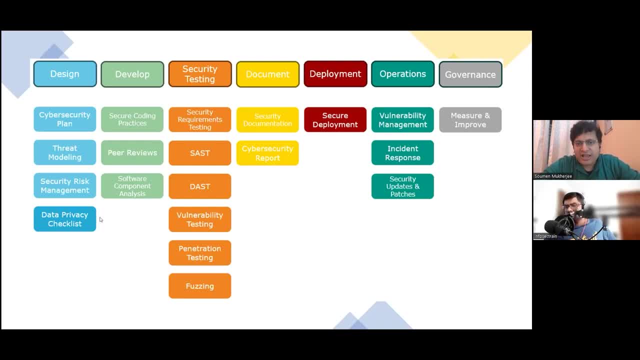 called sam, who has been all that that we can use to measure exactly exactly. we have that. uh, i purposely did not really relate it it right now because i just wanted to keep it more general for people to understand. but, yes, for people who want like to do more. 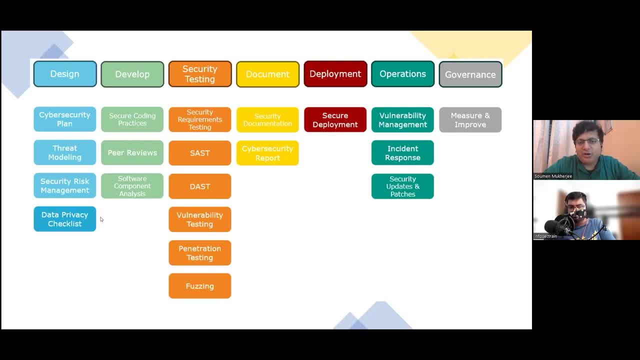 structured approach over sam is definitely a good, very good stat starting point. that's great. so, team, do let us know. like you know, shall we disturb again? uh, sovinda for the new topic, and if you have a question, you can ask me in the chat box and i will be happy to answer your. 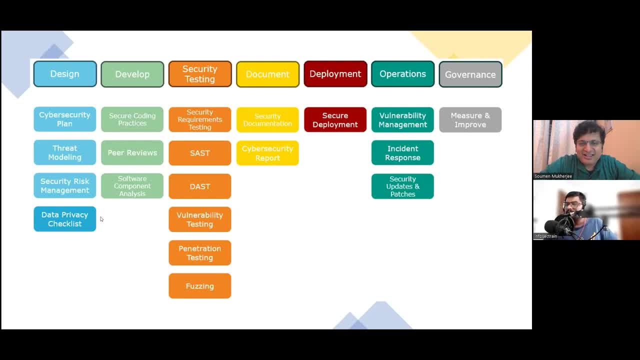 questions. you can share your questions in the comment box, dada, i know, uh, we, i requested you for 30 minutes and it's now been one hour. it is one of the interesting topic, dada, which i am always, you know, amazed to see that. so, dada, there's the last question i want to ask that. 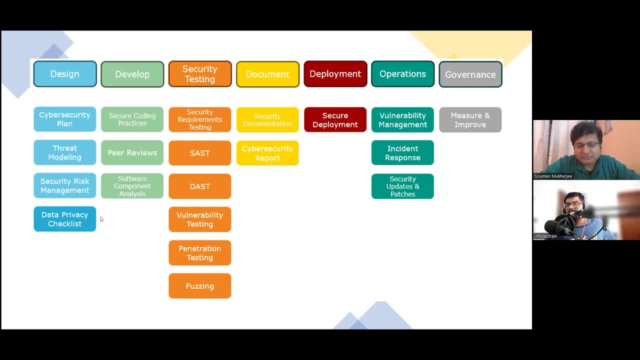 you know, you talk about the processes, you talk about the requirement in each and every stage. now my question is, like you know, do we maintain any kind of like in the company, like if this is basically watched by the person who's beginner and all that, and he 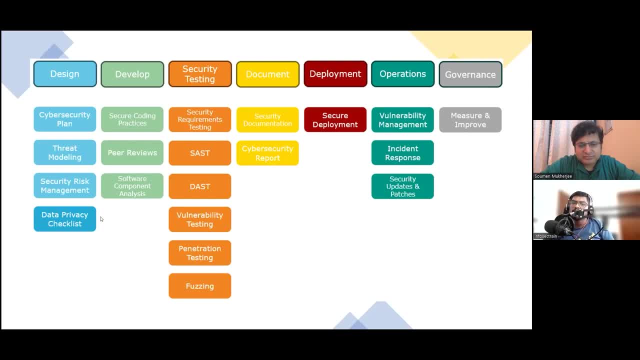 is part of the job requirement or he is part of a job interview that you need to manage as dlc governance and all that. do we maintain any kind of a chat? do you maintain any kind of a document tracker where we make sure you know every product need to go through to this checklist and all that? 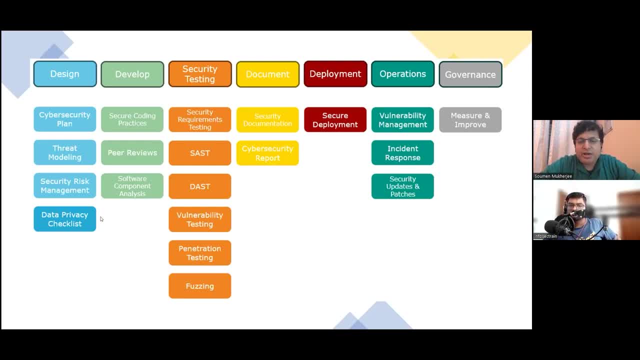 yes, so typically, uh, just like you have a software release process, uh, a software development process. many organizations also have agile development process. uh, there is, there should be a secure software development process also. basically, which says, which typically should say about that: okay, these are the security practices that you should follow as part of the design phase. so you should have a plan, you should. 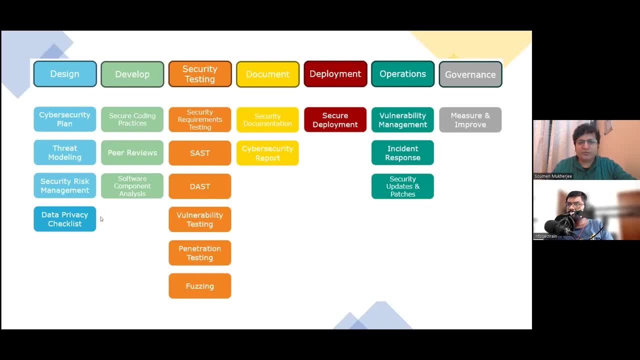 have threat modeling, you should have a risk management session, you should focus on the data privacy and that is how basically a process, typically it can be driven as a process where we say that, okay, from design, development, testing, documentation, deployment, operations and governance, these is all that is required to be done right now, as again, 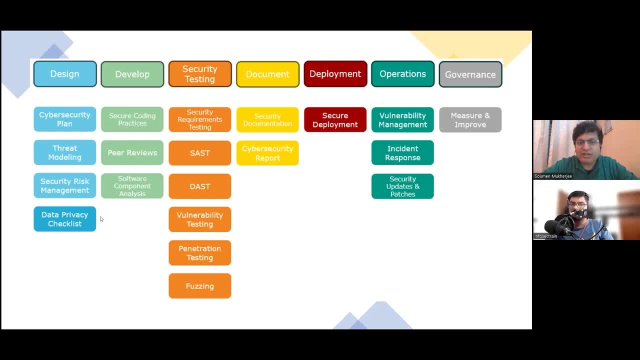 as i said that some say. some people will say, oh, we cannot do it everything at first go, which is fine. you pick and prioritize what you do. it's things to start with, and then you gradually use that measurement and improve on things. but that's great. there is, there is a uh, you know uh, typically for 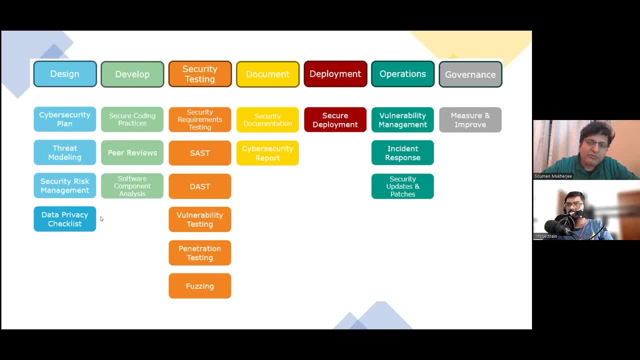 organizations who are matured enough to do that, so that's a good point. i think that's a good point. i think that's a good point. i think that's a good point- and who follow the process models and who have defined processes in place. so there should be a software development, secure software development. 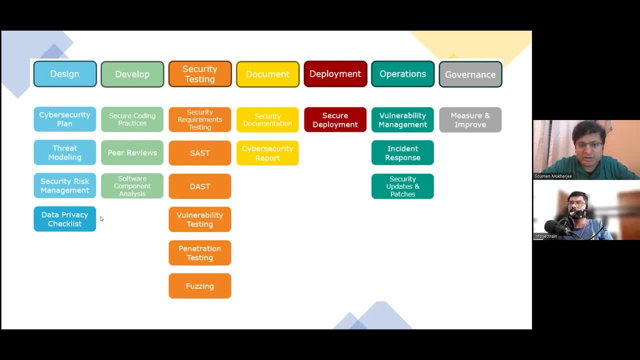 process, also as part of their process documentation. well, that's great. so before we basically wind up the session, you know, do you have any last minute advice? for the freshers who who are looking to these videos and they want to make the journey in security architecture: what is the most important thing they should review? i think the most. 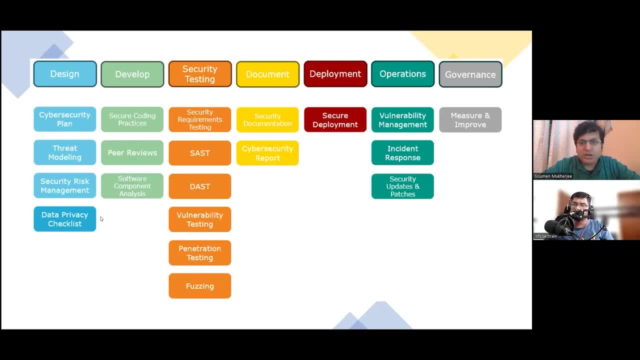 important thing for you when you learn or when you are doing coding, is to also focus on the security aspects of the code that you write. because that is, i think, if you write a code where, let's say, you take an input and you are not doing input validation. 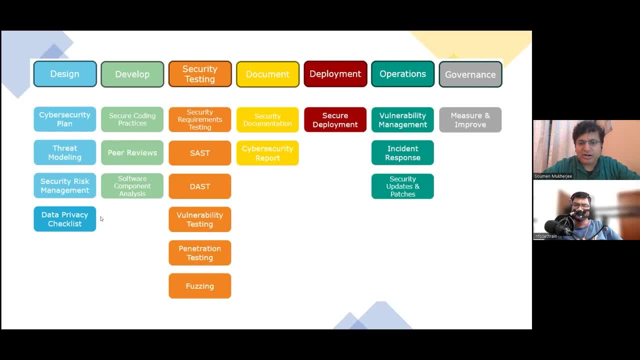 so, basically, you are doing a crime, in my opinion, right, you will basically cause numerous problems down the chain for years to come. so, but as a as a developer, as a freshers who are, who want to, who are going into the industry and say, okay, i like to be a good developer, fine, you, you know code. 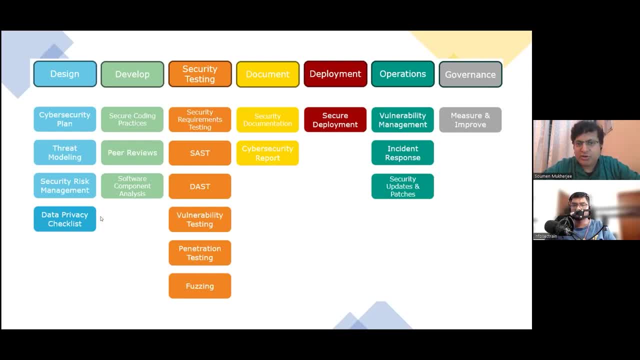 you know technology, you should also know secure coding. you know you should know how to write secure code and you can refer to your ovas secure coding guidelines. it's a pretty elaborate manual that covers all the aspects of secure coding right from. you know input validation to 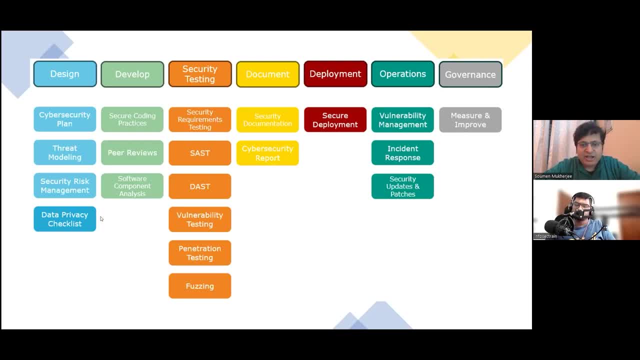 you know sql injection prevention- everything it covers and that is a very good reference for freshers. typically, if you really want to know about secure coding, you prefer over secure coding guidelines. i think that is the best bible that i can suggest to anybody. you don't really need to refer to any other book or any. 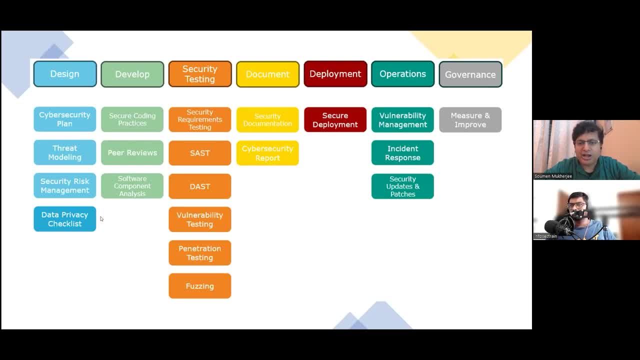 other jargon. just go and look up over secure coding guidelines. i think that is the best thing that you can do. that is that is great, and and thanks for the great insight and truly appreciate, you know, your knowledge that you have shared with us today. Right, it's been a privilege talking to you, Prabh, you know, i think, because the kind of things 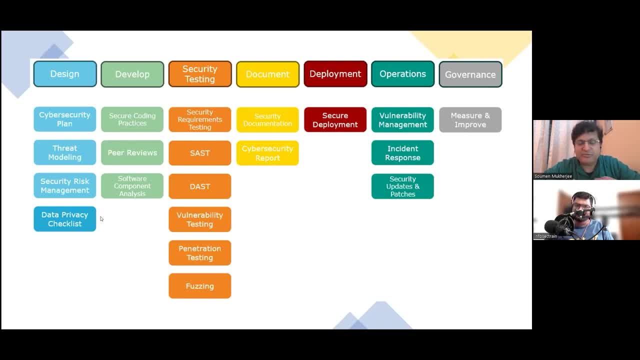 that you have a vast experience. you know we really do look at the small things, but you look at and our world of things and so the kind of questions that you put up, they were very, very good and very insightful. you know that. also, as i said earlier, that i will take 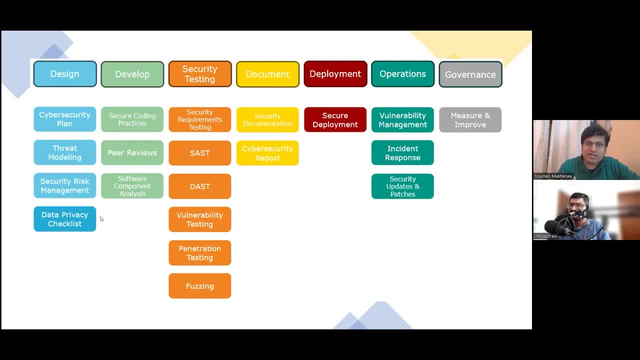 away a lot of learning also from this session and you know those questions have been all very good, been really truly in that sense, uh, been my learnings for the session. that, okay, you know that typically, yes, like the kpis thing, yes, the measurement, the process thing, you know how to. 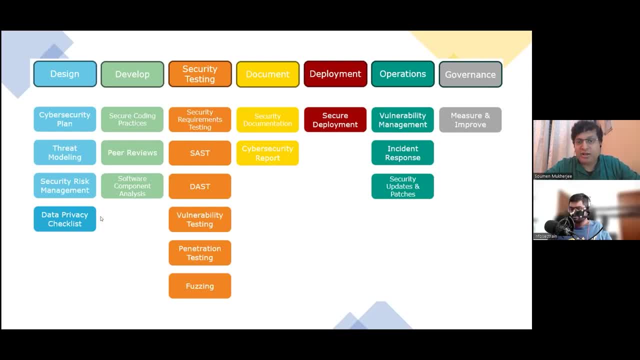 document it in a more formal way. i think these were something that were an even an eye-opener even for me. that that is a quality i like about you. know you don't take that, the things on head, that that is that is why you're well grounded and that is how you you carry your aura. don't go by his statement. 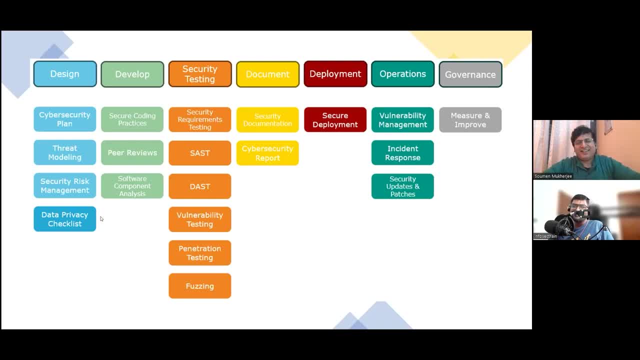 guys, he, i know him, he's uh, you know the kind of a discussion he used to have in product. so it's really well. i think it's a i i think it's been a privilege actually. you know, i mean i've worked with people who have been pioneers in the industry of security. you know you talk about your. 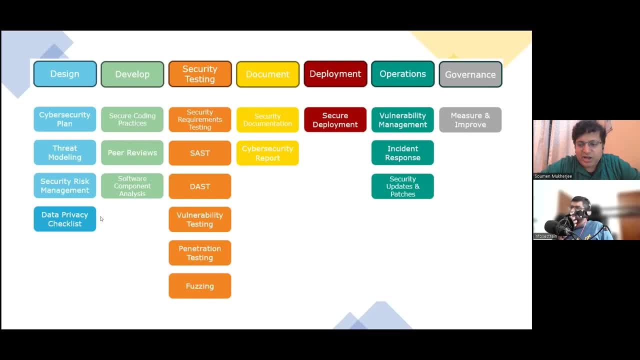 you talk about your neft things, your imps, money transactions, what that is happening. i've worked with people who have actually developed those technologies which are being used today in the industry to safeguard things. i have worked with people who are, who have been, who have written the ipsec protocol, which is the underlying foundation of 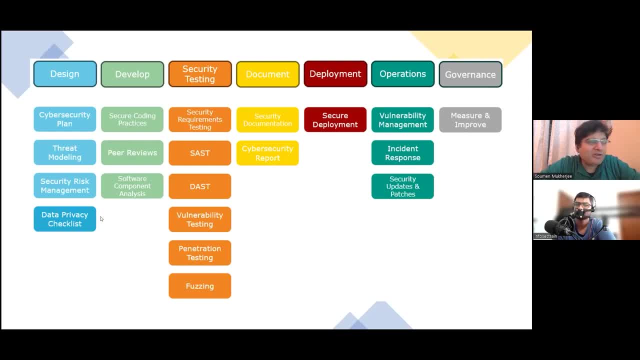 the ssl vpn which is used for, you know, remote work. so i it's, i think i've been fortunate enough in that sense and, uh, you know, i just try to make sure that what i understand, i understand, that conceptually, i really grasp the concept and you know, then i think it becomes very easy and learning. 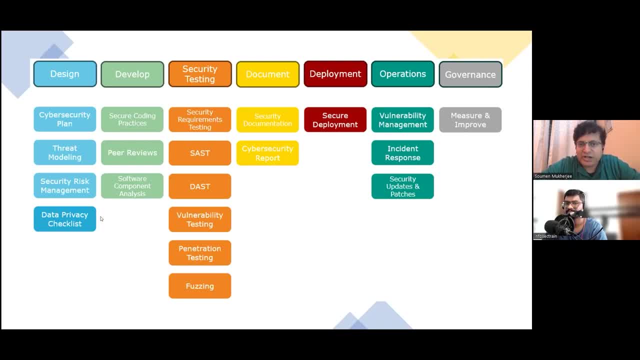 is a is a continuous journey. it's something that you do every day, every time, uh, and there's no end to it. so, you know, i think that is that is the key to all this. thanks, thank you, thank you, thank you so much, and i really, i know, i, i really take, i am, i'm going to have a very good insight and i'm 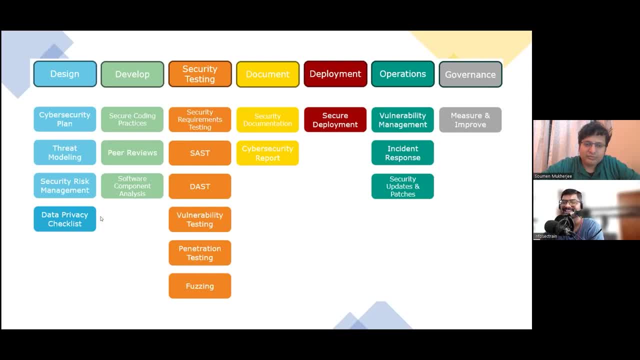 i'm planning to make one video and i'm going to use this particular uh slide on that. i'm definitely give you credits because you deserve that, because i got some new insight about governance, which i was having a limited visibility because for me the requirement was the first, and then design. but yeah, it makes sense. see, when i speak to the, the guy who work. 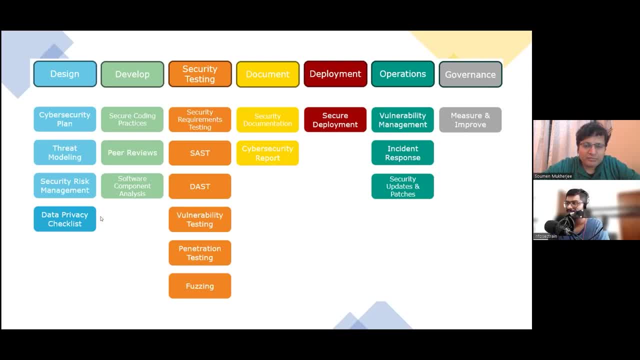 on the industry, the work on the ground. they don't work on theory. right, you're getting a point. so i come for the session. i say the first stage is basically design, then we develop and i gone after fifth day. so main in front of customer cannot say 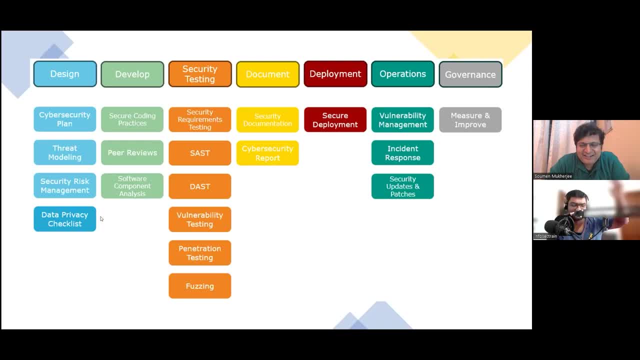 okay, we'll have a design, and then we have a development. sorry, we have a requirement, then we design. boss, okay, you're telling me: uh, on on paper, please execute that. and this is where the reality comes. so for me, the new insight i got is the most important part is a design development. 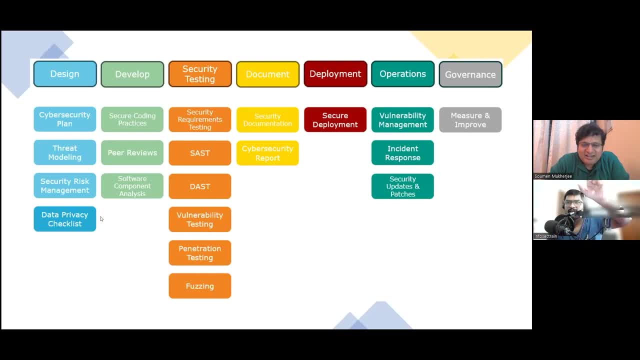 which is a shift right bottom approach, which is a very good point, and i'm sure i haven't seen any videos which talk about this level of sdlc from a product security perspective and i'm sure this, this video, going to rock and team trust me, do let me know should i disturb him. 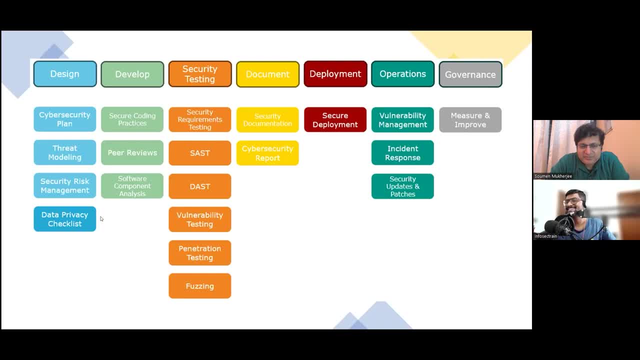 again, because see people sit on a gunpoint. they say so. for me the gunpoint is like live, live camera, okay. so always welcome, always welcome. it's, it's a privilege actually. uh, you know, it's a. i really appreciate, uh, this kind of interaction, because this is where you can actually you have the